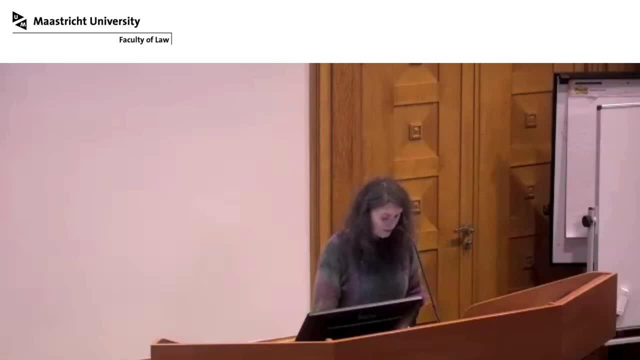 hall. Joanna will introduce us to access to justice in environmental matters- a key topic in environmental law- And she will focus on access to justice at EU level. Dear Joanna, you can take the floor. Good afternoon everyone. It is a great pleasure to join you online for this. 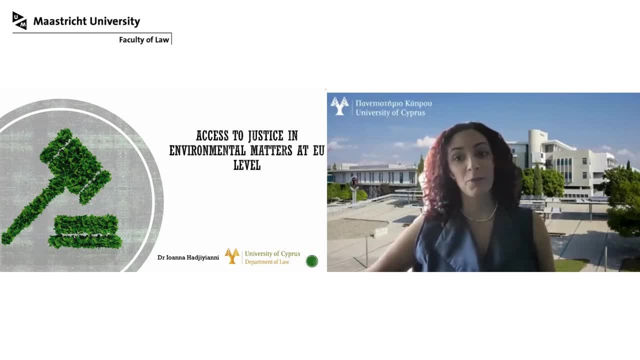 environmental law lecture series. Firstly, I would like to thank Professor Peter for the kind presentation to deliver this lecture on a topic that I have long found fascinating and in which developments are always ongoing and topical. This lecture examines the scope of access to the Court of Justice of the European Union in environmental matters for challenging the legality of 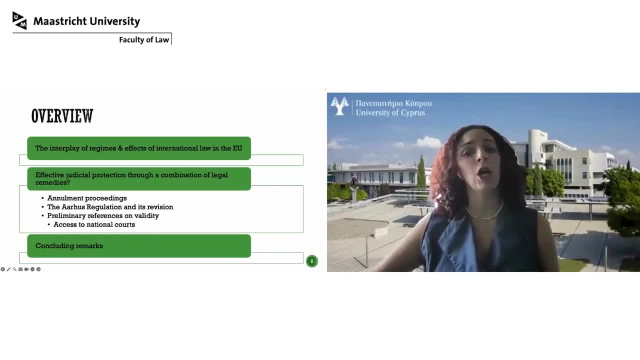 acts adopted by EU institutions and bodies. My talk will start by setting out the interplay between EU law, particularly the Aarhus Convention, and EU law, focusing on the role of the Court which determines the internal effects of international agreements. Now the presentation examines the 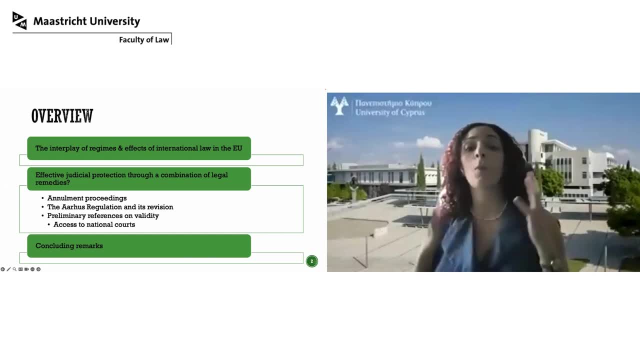 effectiveness of judicial protection in environmental matters, which is meant to be ensured through a combination of remedies which together provide a complete system of remedies. In examining the different legal remedies, I will be focusing on issues of standing, which ultimately determine who has access to the legal system. I will also be talking about the role of legal 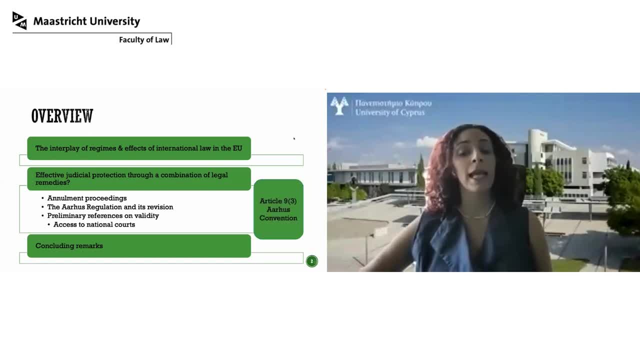 law in the implementation of the Aarhus Convention. In this context, I will be drawing attention to the impact of Article 9 of the Aarhus Convention, which is limited in determining access to the Court of Justice directly under an amendment proceedings, but has influenced the revision of. 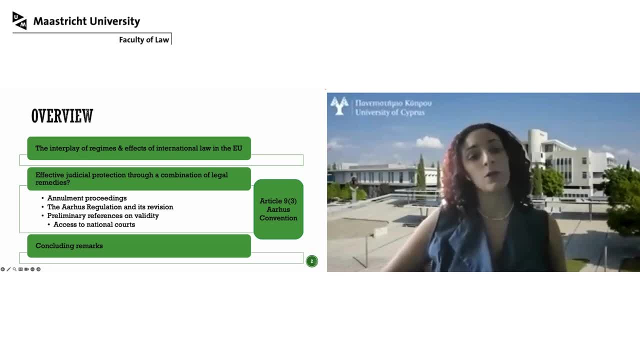 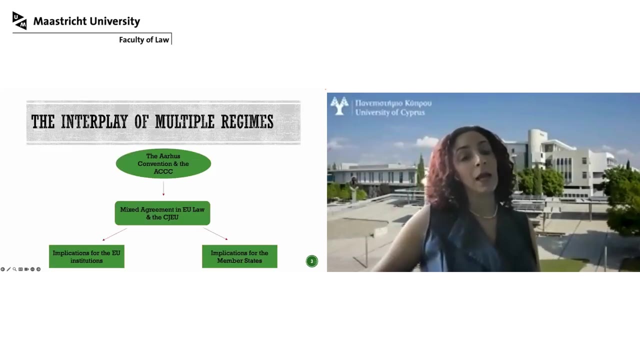 the Aarhus regulation. In the EU legal order, much emphasis has been placed on indirectly accessing the Court through preliminary references by national courts. but this depends on actually having access to national courts in the first place. Now, at the international level, the Aarhus Convention adopted in 1998 under the 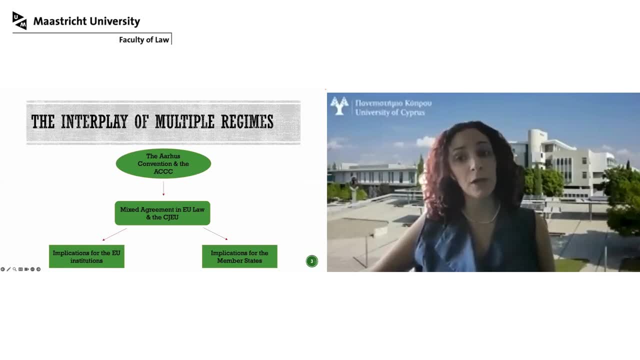 auspices of the United Nations Economic Commission for Europe, sets out general obligations for ensuring access to environmental information, public participation and access to justice. Compliance with these obligations is overseen by the Aarhus Conventional Compliance Committee, which is an innovative compliance review mechanism before which members of the public 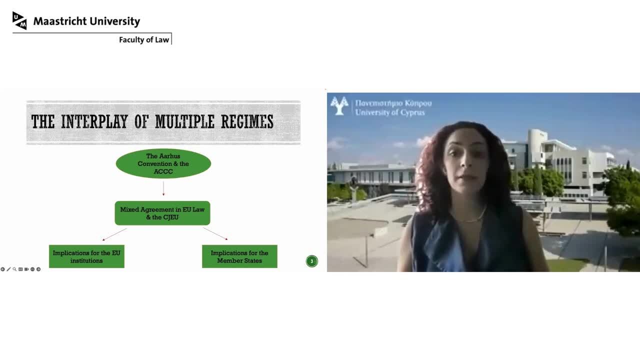 including NGOs and other contracting parties, may bring complaints. Since the establishment of the ACCC in 2002, it has issued a significant number of findings, including on the Convention's circular on access to justice When we get to the EU legal order, depending on the situation, EU environmental law. 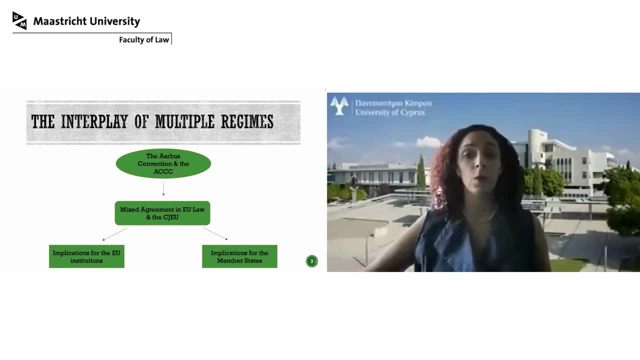 and the EU's current policy may be violated by EU institutions, For example, when the Commission authorises an active substance to be used in pesticides or, on the other hand, by national authorities when they authorise the construction of polluting. 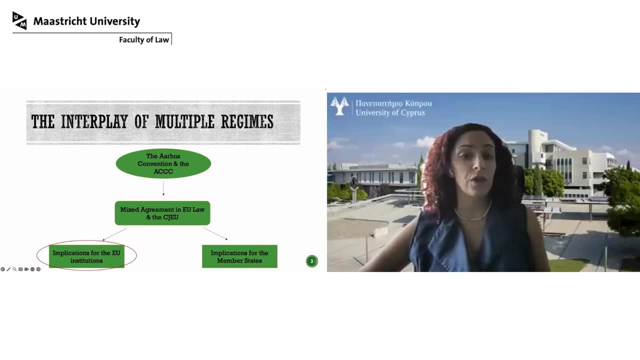 industries in protected areas, for instance. Now, under EU law, the Aarhus Convention is considered a mixed agreement. It indicates that both the EU itself and the 27 member states are contracting parties, And the court has confirmed that it has jurisdiction to interpret the Convention. 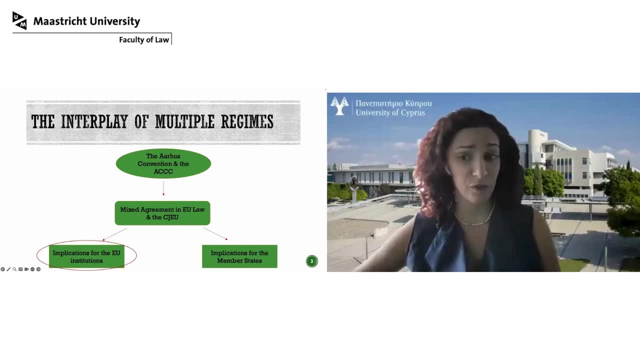 on Access to Justice, also for the member state, and even in relation to Article 9, 3,, which is a provision that can apply in situations falling within the scope of national law and to situations falling within the scope of EU law. The focus of today's lecture will be啊. 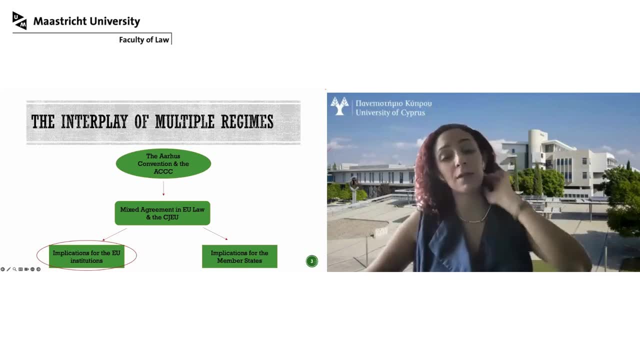 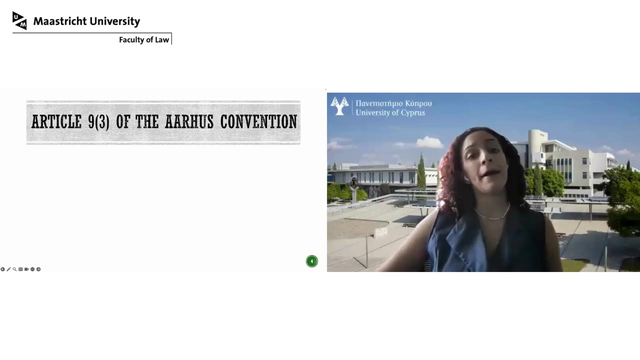 indications of the provisions on access to justice, particularly Article 9.3, for the EU institutions and access to justice at the EU level, Starting from the relevant provision of the Aarhus Convention. Article 9.3 establishes a general right to access to justice in the sense that it does not depend on the other. 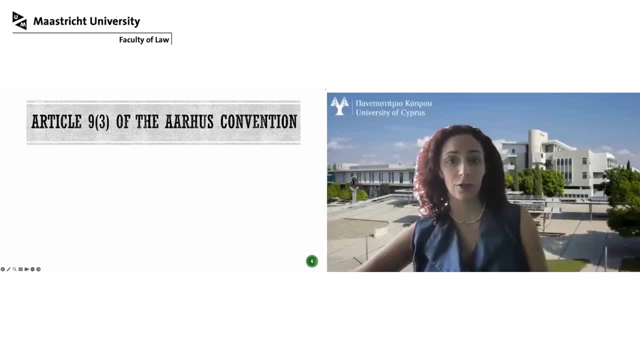 two pillars on access to information and public participation. Now, what does Article 9.3 require? It requires parties to ensure that members of the public have access to judicial or administrative procedures to challenge violations of environmental law. And perhaps the most important and controversial aspect of Article 9.3 is that it allows certain 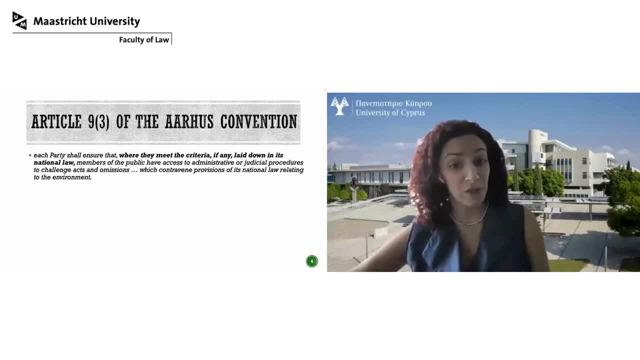 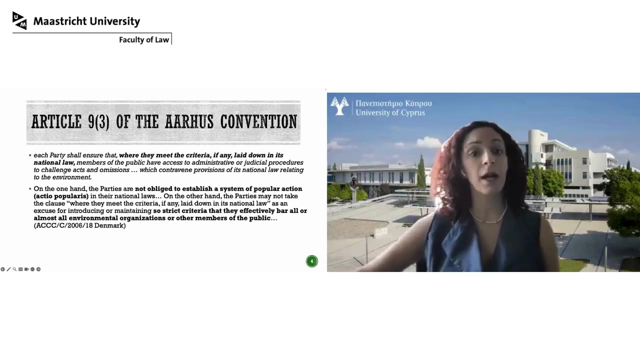 discretion to parties to set criteria usually relating to status. There are certain discrimination requirements that are called the Commission Act, and those are not sufficient in order to be following the international law which may qualify such access. Now the ACCC, in findings against Denmark, has clarified that Article 9.3 does not establish: 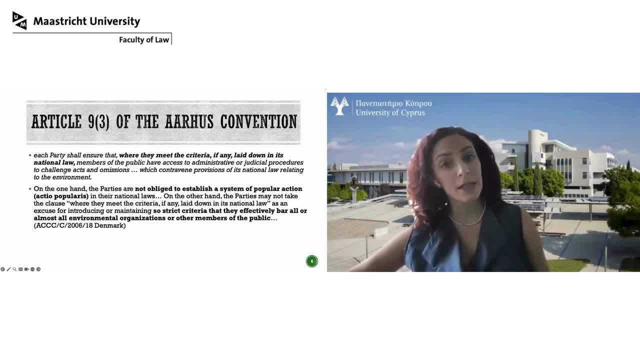 actio popularis, in the sense that anyone can have access to courts, but at the same time it does not allow parties to establish criteria that are so strict so that effective negotiation is possible. with an exception of the commission on access, they bar all, or almost all, environmental organizations or other members of the public. 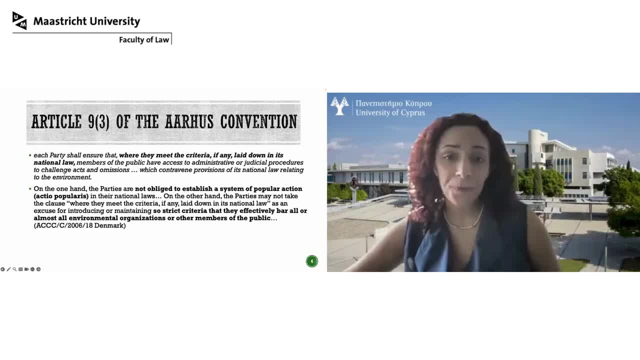 from having access. This reflects the underlying rationale of the convention, which is to guarantee access to justice, and which the parties need to take into account when they set criteria in their national laws. Now the requirements of article 9.3 are supplemented by article 9.4, which requires: 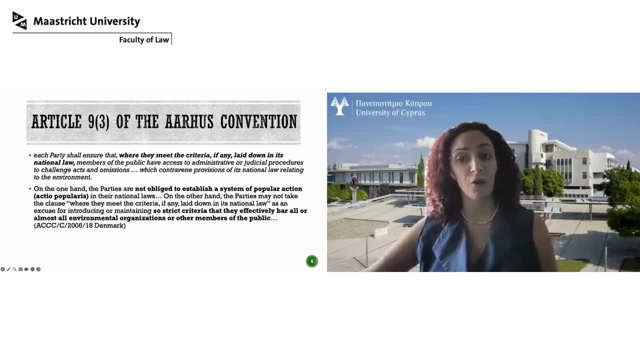 procedures under article 9 to provide adequate and effective remedies, as well as be fair, equitable, timely and not prohibitively expensive. In this context, the ACCC issued findings against the European Union, initially in 2011 and finally in 2017, for failing to comply. 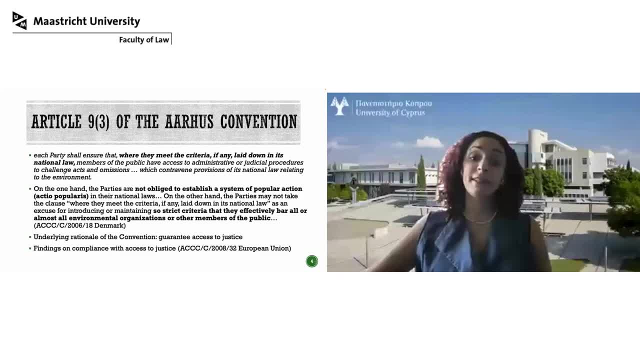 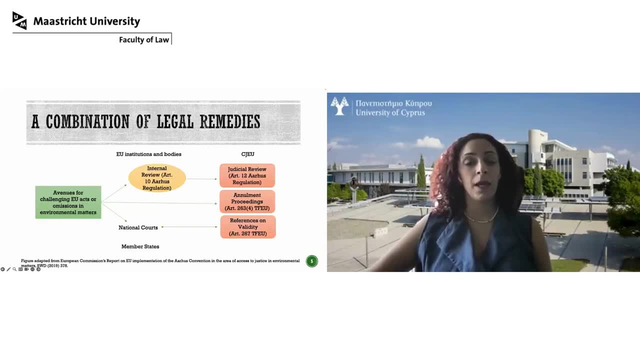 with the requirements of article 9.3 and 9.4. despite the multiple remedies provided for in EU law, In the European legal order there are multiple avenues for putting article 9.3 into effect which are meant to work in combination like pieces to a puzzle to create. 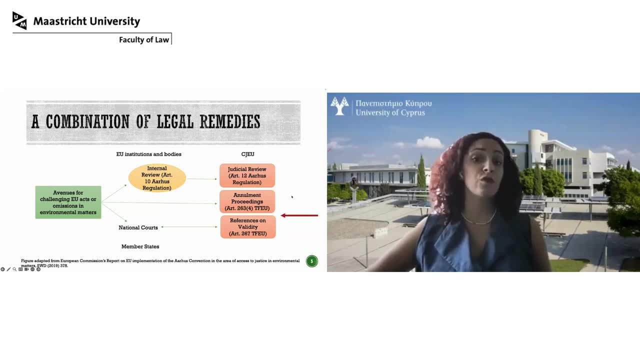 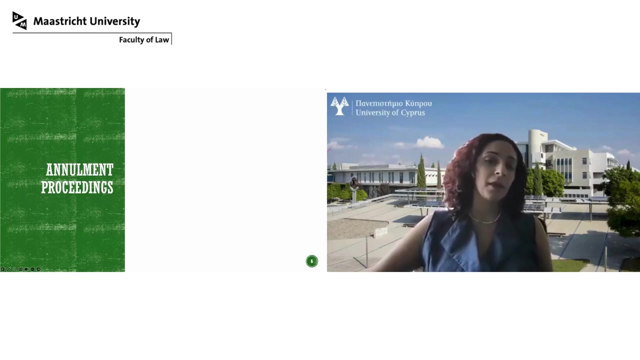 a complete system of remedies. The first, most direct way of having access to judicial review before the court of justice is provided under article 263. Paragraph 4 of the treaty on the functioning of the European Union, and it is also the most restrictive Standing requirements for non-privileged applicants. that means members of the public and 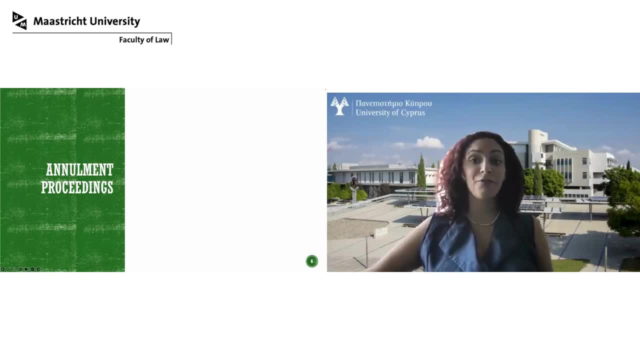 NGOs under article 263.4 have been interpreted narrowly Particularly. the requirement of individual concern, as the article says, has been consistently interpreted since 1963 in the common case in a restrictive manner which essentially requires an applicant to be affected in a way that differentiates them from all other persons, just as in the case of the person to which 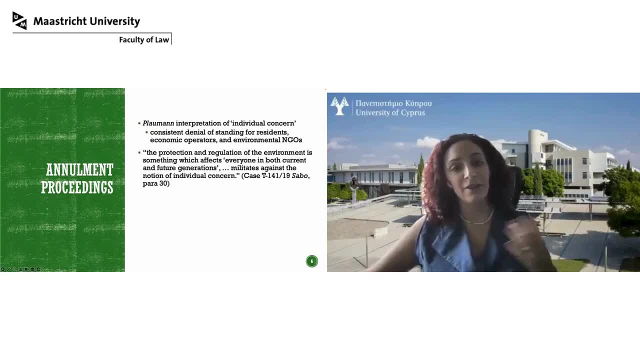 a decision is addressed. You can imagine that in environmental cases, where affected interests are usually of collective nature, this has led to different kinds of actors systematically being denied access to the court under article 263.4, and they do not usually form part of the closed predetermined class, and this includes economic. 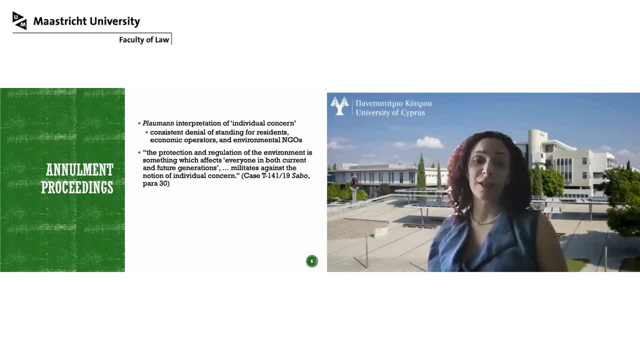 operators, residents in nearby areas of polluting activities and NGOs. This approach was recently reaffirmed by the court in the case of Sabo, a case concerning an annulment proceedings against the EU's climate mitigation action, Confirming in this case that individual concern. 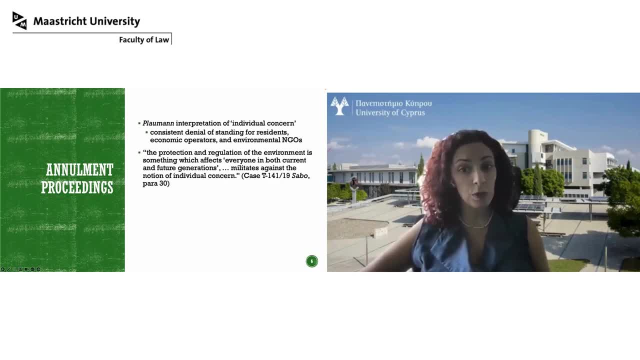 is a test of intensity and not scope, essentially saying that the larger amount of people affected, they are less likely to have access to the court under article 263.4.. Here we have a mention of intergenerational equity, basically the fact that the protection regulation of the environment says: 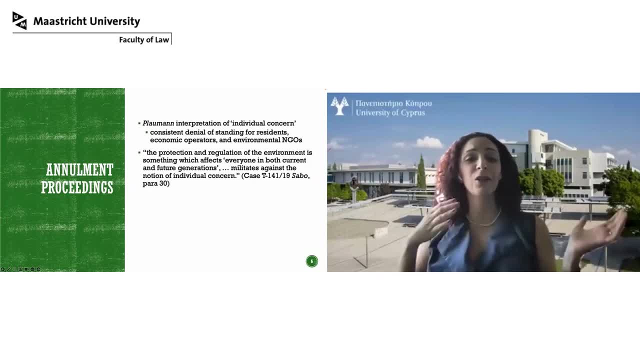 the court affects everyone, in both current and future generations, actually works against the notion of individual concern. As a response to some of the gaps created by the restrictive application of individual consent, a new avenue for direct access to the court was created by the Lincoln Treaty. 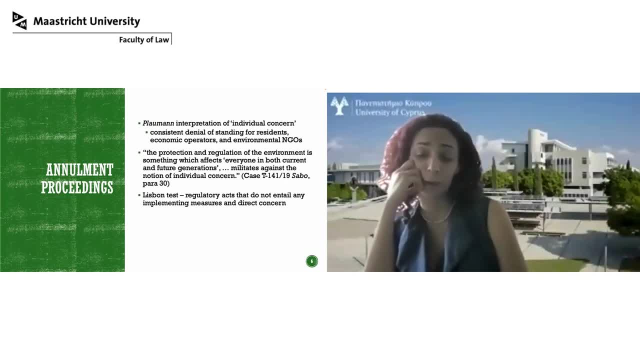 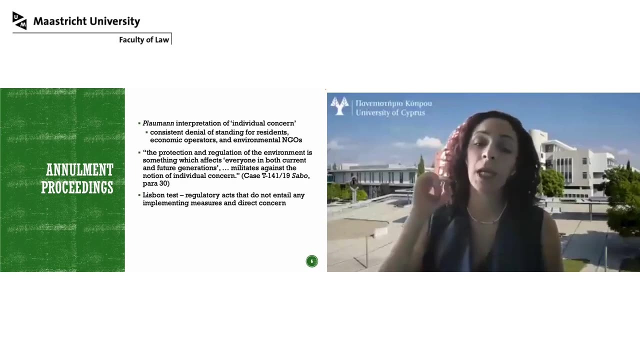 in the third link of Article 2634.. So this establishes access to the court to non-privileged applicants when they are directly consented by regulatory acts that do not entail any implementing measures, And it has been interpreted to cover only challenges to acts of general application. 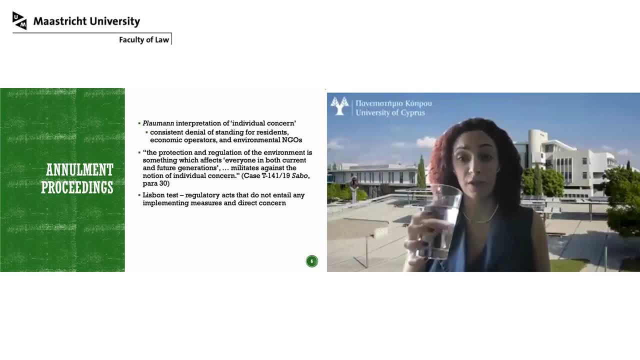 that have not been adopted through a legislative procedure, and only in situations where there is absence of any measure by the Member State to put the regulatory act into operation, even of a mechanical measure In relation to environmental cases. the Lisbon test has not significantly altered the position. 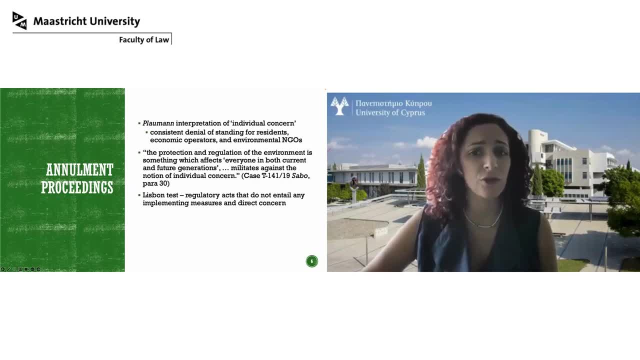 of individuals and NGOs. Most environmental measures would not qualify as regulatory acts not entailing implementing measures. Most environmental measures are directives which by nature often entail discretion and always require implementing measures. In any case, applicants still have to demonstrate direct concern under the Lisbon test. 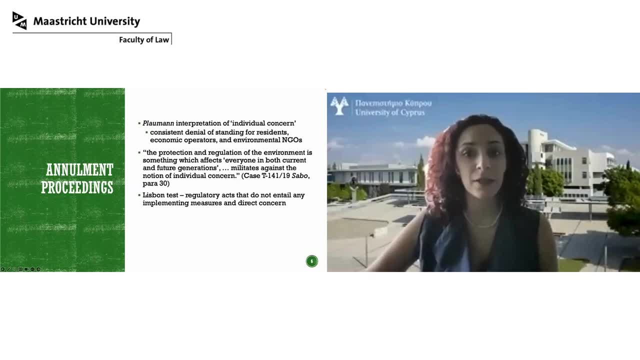 This requires the legal position of the applicant to be directly affected, Given the discretion embedded in environmental measures, and that the damage caused may not be the direct result of EU action, applicants in environmental cases still face considerable obstacles. In the Sabo case, for instance, the damage caused to the applicants as a result of cutting. 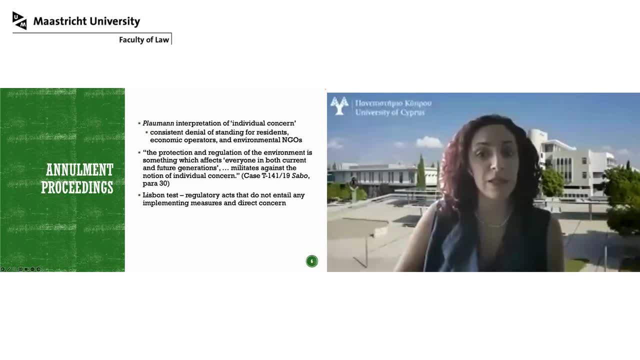 down trees would not be directly affected. It would be unlikely to be deemed a direct consequence of the EU's rules on the use of biomass, given the multiple causal events between the EU Act, the Member State's action to meet renewable energy targets, the increased demand for pellets and the ultimate result. 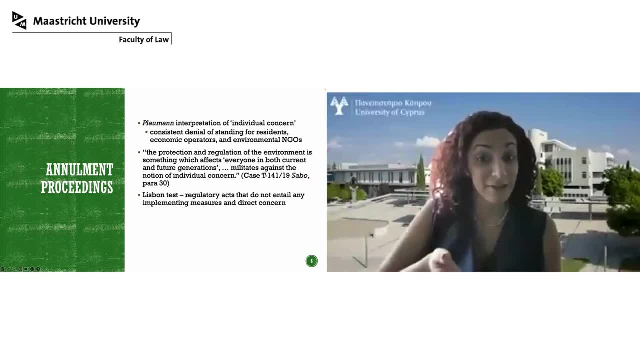 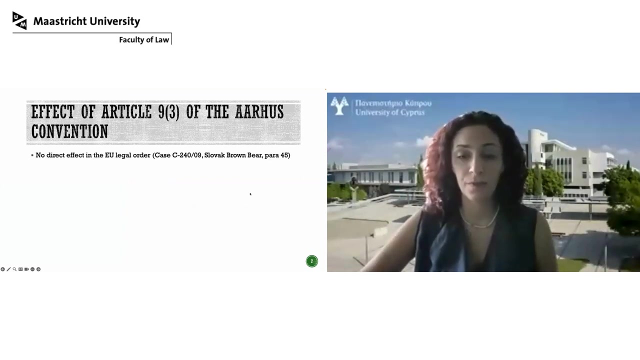 on cutting of trees in the area where the applicants live. Overall, different strategies have been used by individuals to address environmental issues. The Key Advantage of the POC was to see if the EU could simply change its approach to environmental cases. Among these failed strategies is the attempt to use Article 9 of the Aarhus Convention. 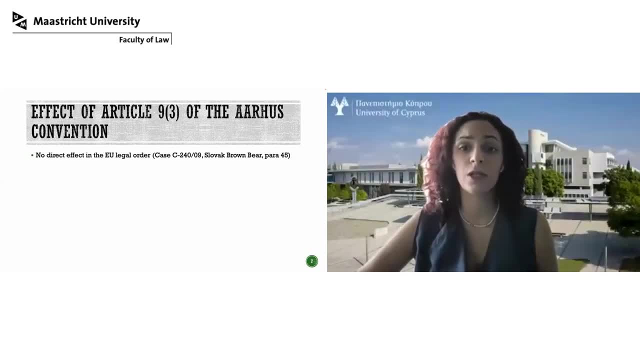 Article 9 has no direct effect in the EU legal order, since the court- in the sense of applicants being able to rely on it directly as a legality-based engagement- The Court of Amnesty has refused to let the EU have the court's access to the legal procedures. 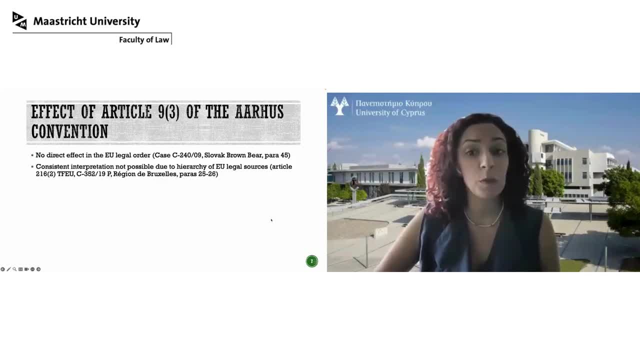 for any of the Virgil and Zayn transactions. The Court has determined that the EU's legal practices should not be restricted to one environment. Second, we have seen a number of US states and state institutions have not yet reached an agreement with the EU to not be required to use this measure. 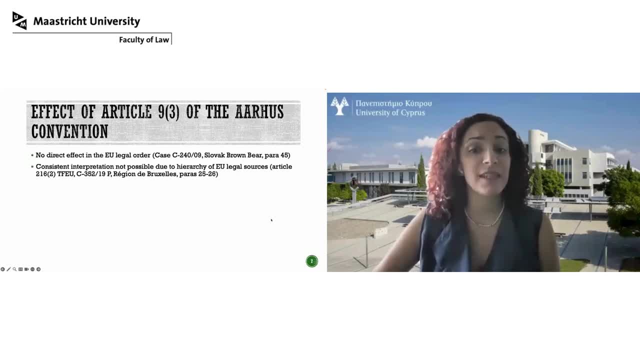 Article 93 into account by consistently interpreting Article 234.. According to EU law, established EU law, international agreements concluded by the Union bind the institutions and prevail over acts of secondary EU legislation, but they do not have primacy over treaty provisions And, in any case, the Court considers that Plowman is simply the criteria. 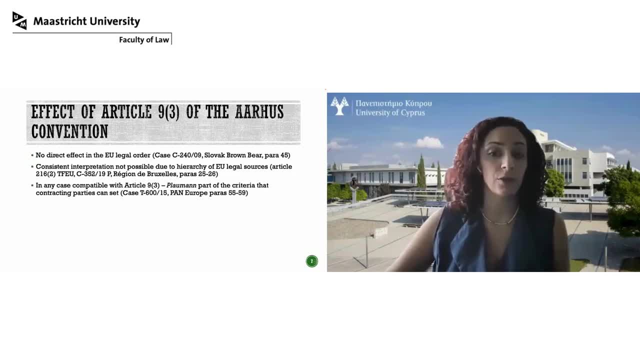 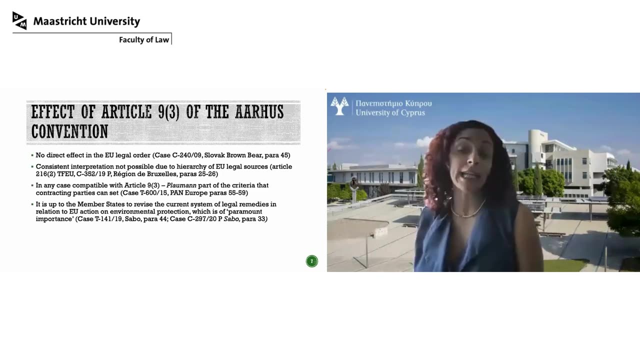 that the EU has decided to lay down, as permitted by Article 93.. In Sabo, the Court concluded that, despite the paramount importance of environmental action and the fact that a different system of remedies could be envisioned for challenging the legality of EU action on environmental matters, it's up to the Member States. 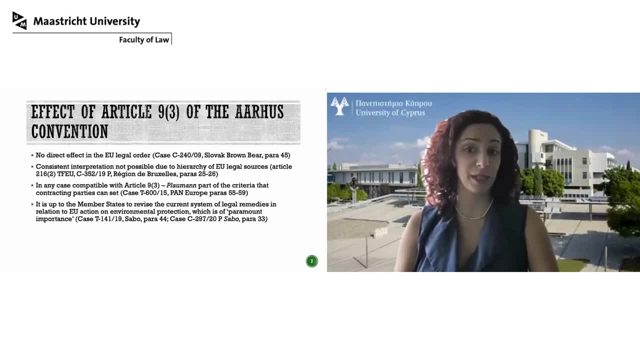 to revise the Act. It's up to the Member States to revise the treaties and not for it to change its interpretation, So shifting the responsibility to the drafters of the treaty, potentially to create a separate environmental avenue for directly accessing the Court. 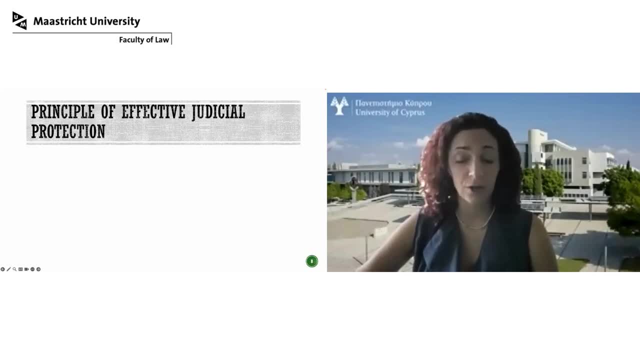 Apart from Article 93 of the Aarhus Convention, attempts to rely on the principle of effective judicial protection under EU law, including its recognition in Article 47 of the Charter of Fundamental Rights, have also failed, with the Court stressing again the hierarchy and importance of following the treaties. 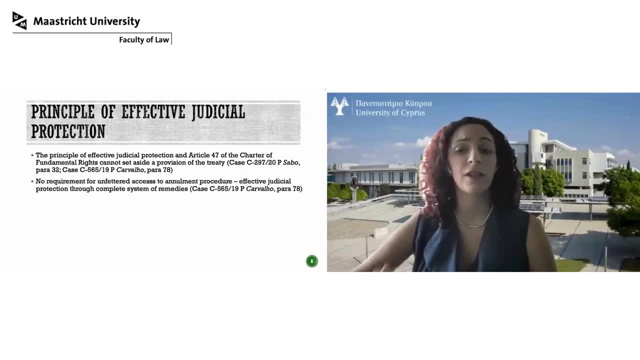 In any case, in the eyes of the Court, effective judicial protection does not equal unfettered access directly to the Court, but it is meant to be ensured through a combination of the two. In any case, in the eyes of the Court, effective judicial protection does not equal unfettered access directly to the Court, but it is meant to be ensured through a combination of the two. 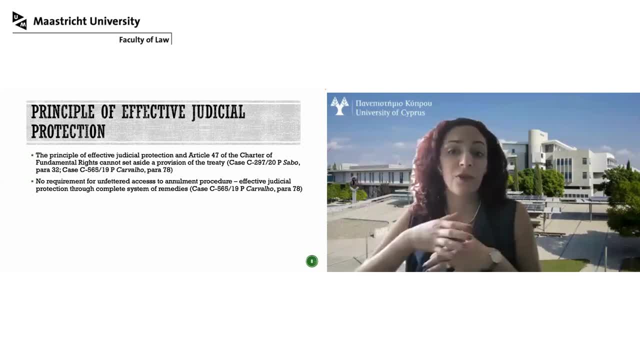 In any case, in the eyes of the Court, effective judicial protection does not equal unfettered access directly to the Court, but it is meant to be ensured through a combination of the two, Considering the announcement proceedings only to be one piece of the puzzle, 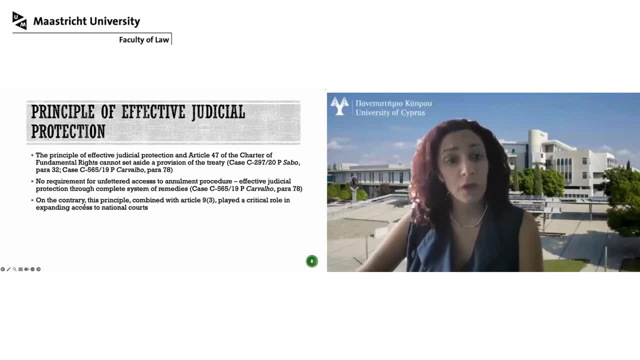 Considering the announcement proceedings only to be one piece of the puzzle. On the contrary, the principle of effective judicial protection- in combination with Article 93, has played a crucial role in the Court's case law on access to national rapports, and we'll come briefly back to this differentiation, which can be problematic. 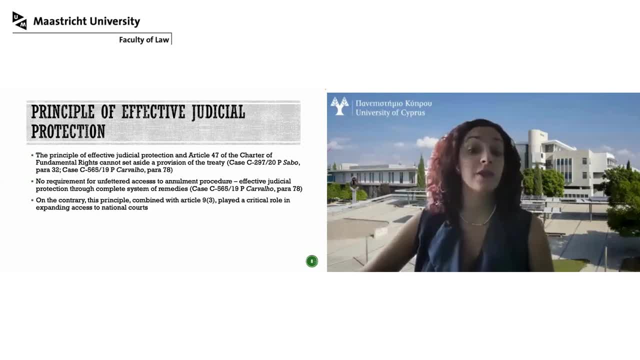 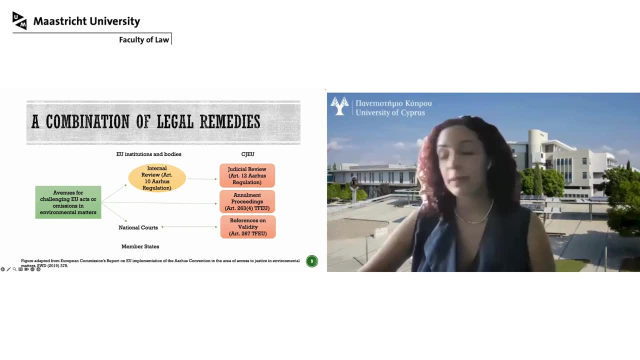 towards the end of the presentation And we'll come briefly back to this differentiation, which can be problematic towards the end of the presentation, Given the limited access, especially that environmental NGOs have to run on proceedings. one of the main alternative avenues for access to justice for this type of applicants has 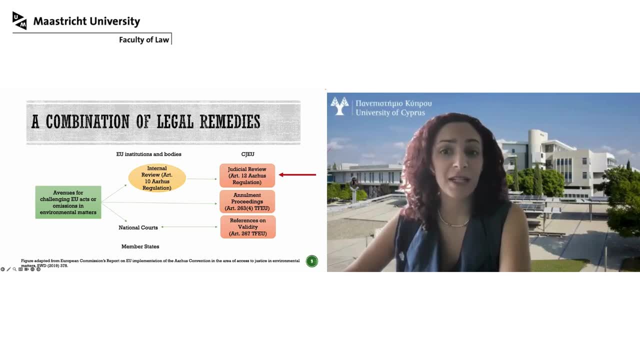 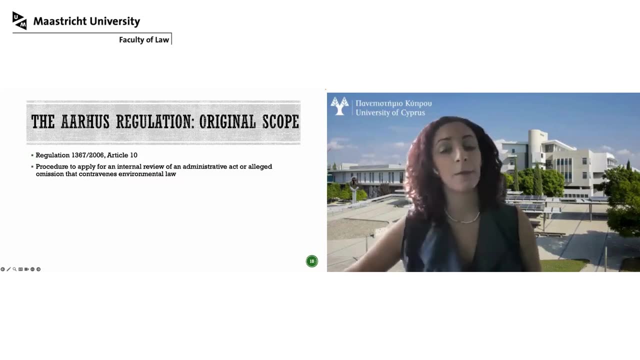 been an administrative review procedure provided under the ARHUS regulation. Rule 10 established the procedure to request an internal review of administrative acts or permissions that contravene environmental law. Now, this is inherently of a different nature, because the request for internal review is. 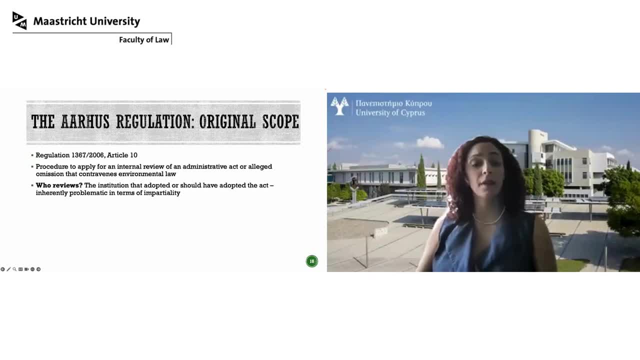 lodged with and examined by the institution or body that adopted or should have adopted a specific act. So the review mechanism inherently raises the question of whether the internal review is valid or not. Does this consent as to the impartiality, adequacy, fairness required by Article 9 of 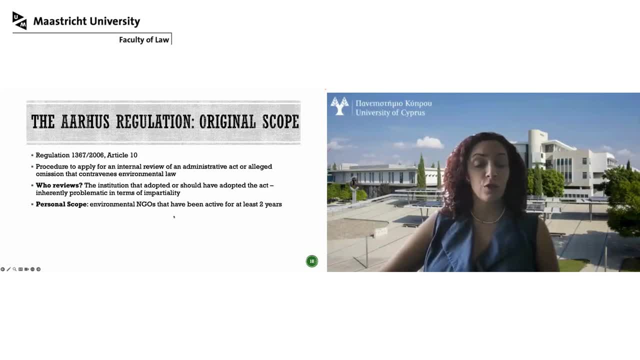 the Convention. In terms of its personal scope, the initial version of the ARHUS regulation was very limited Only to environmental NGOs that had been active for at least two years in a Member State, And, in terms of its material scope, it excluded both legislative acts and measures of law. So it was a very limited version of the ARHUS regulation And, in terms of its material scope, it excluded both legislative acts and measures of law. And, in terms of its material scope, it excluded both legislative acts and measures of law. 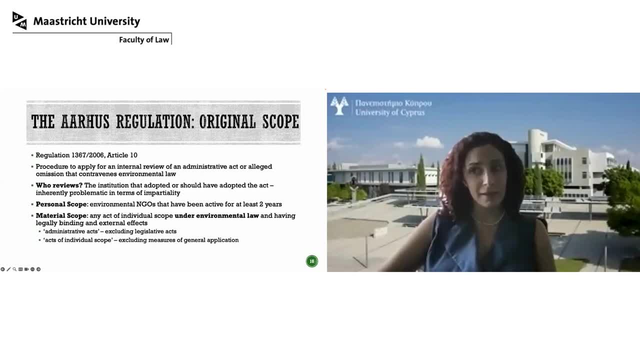 And, in terms of its material scope, it excluded both legislative acts and measures of general application. In practice, since its entry into force, 80% of the requests lodged with the Commission were found inadmissible And, from this, more than half of the requests made to the Commission were rejected because 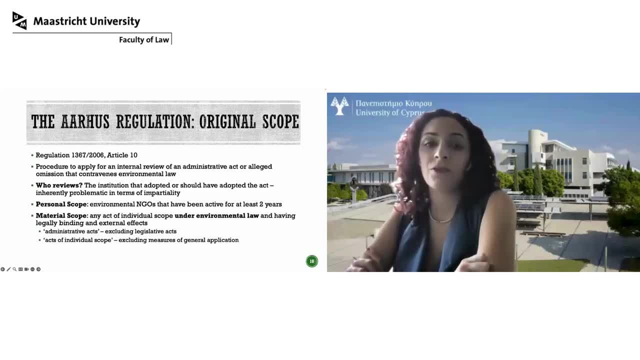 they were not considered to be of individual scope. So, for example, it excluded acts addressed to the Member States, such as acts addressed to the Member States, such as acts addressed to the Member States, such as acts addressed amending maximum residue levels of pesticides, and commission decisions authorizing 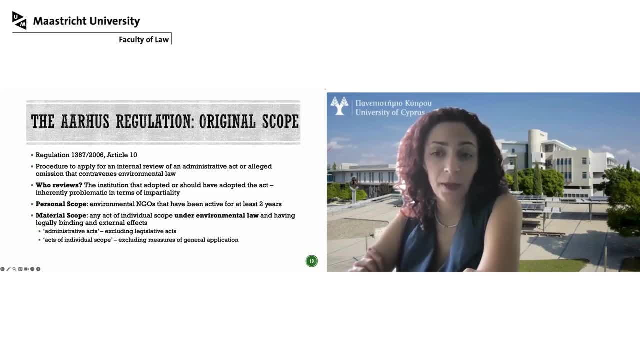 derogations from the Equality Directive, A very small number was considered admissible, for example concerning authorizations of placing on the market of genetically modified products and chemicals. but even those requests that were deemed admissible by the commission, they were found not to violate environmental law and usually this was on the basis of a very 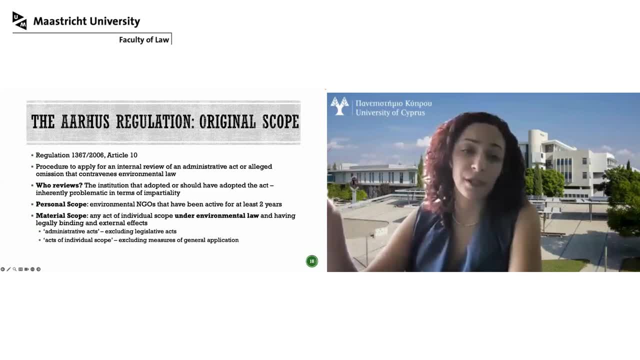 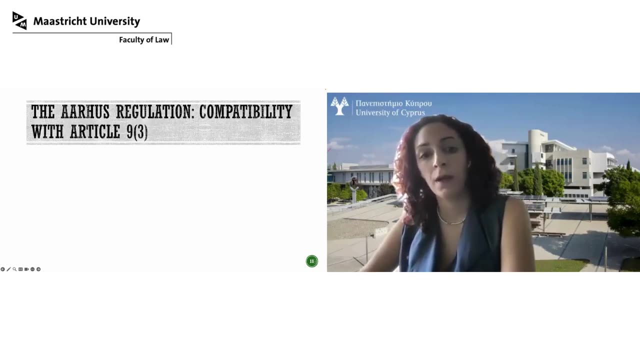 brief statement by the commission, disagreeing with interpretations suggested by the NGO that lodged the request. In fact, none of the requests lodged with the commission have led to an act being revised or withdrawn. You can imagine that the material scope of the Act's regulation was: 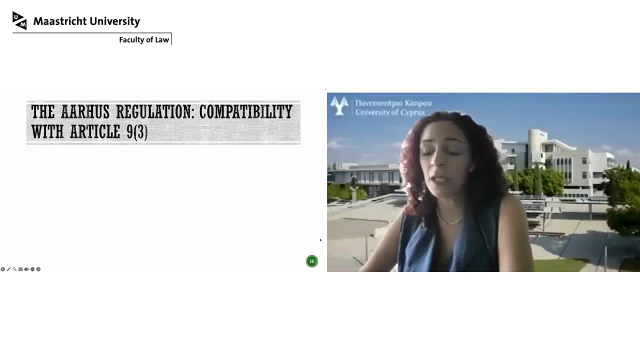 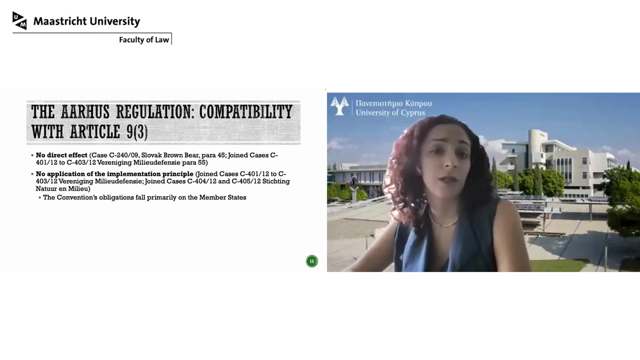 challenged before the Court of Justice. As mentioned already, Article 9 does not have direct effect, which means that it could not be used as a legality benchmark directly for reviewing the regulation. The Court also refused to apply the so-called implementation principle that would have allowed a legality benchmark. 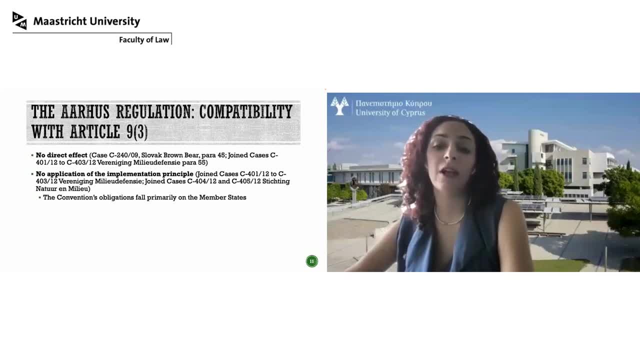 This principle was developed in relation to WTO agreements which do not have direct effect on the EU legal order. According to this principle, it is possible to review the legality of EU law on the basis of an international agreement which does not have direct effect, when the EU Act at issue explicitly refers to provisions of the agreement. 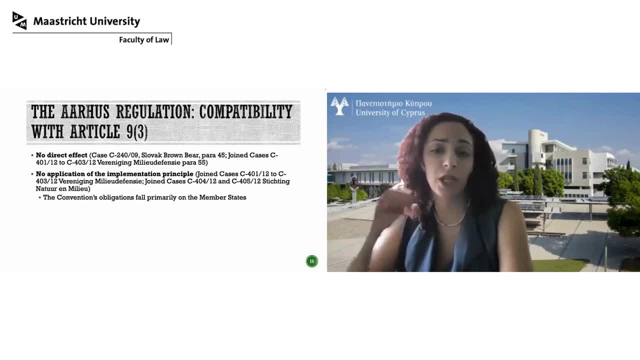 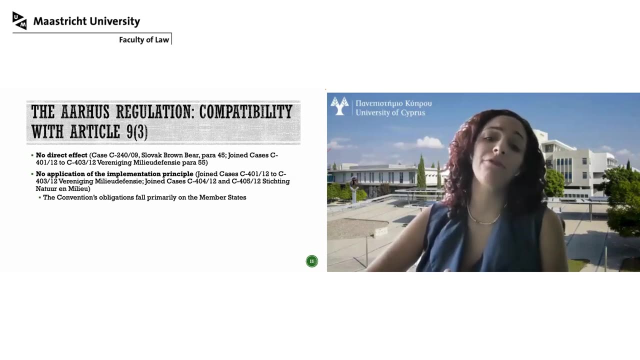 or it tends to implement a particular obligation of the EU Act. In refusing to apply this principle to the Act's regulation, the Court emphasised that the Act's Convention's obligations primarily fall on the Member States and any gaps in judicial protection should be filled at the national level. It was also not possible to broaden the scope of the regulation. 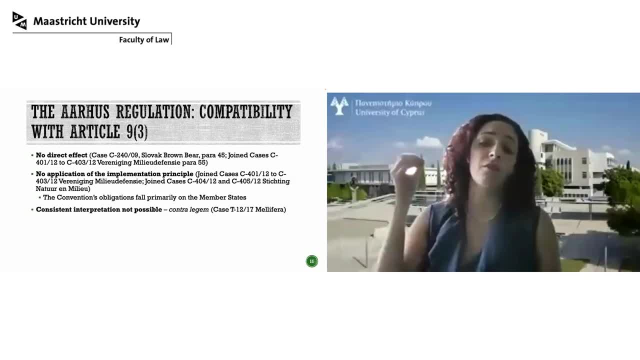 through consistent interpretation. The Court says the regulation explicitly provides that acts are reviewable under the regulation have to be of individual scope. Interpreting this in a different way would amount to contra-legal interpretation, against the letter of the law, and was not possible. 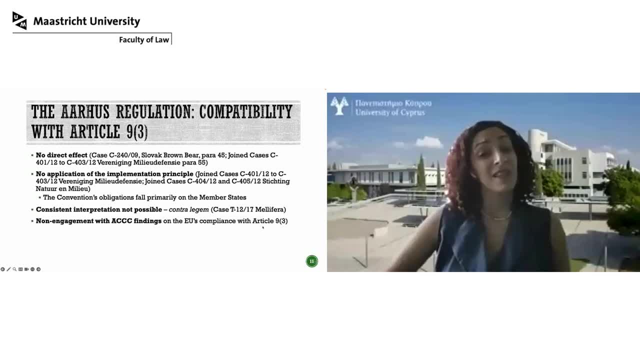 through judicial interpretation. Interestingly, the Court did not explicitly and meaningfully engage with the ACC findings on the AHU's regulation, which clarified that, yes, we do have a caveat in Article 9 allowing for criteria to be imposed, but this does not leave discretion as to the kinds of acts that may be. 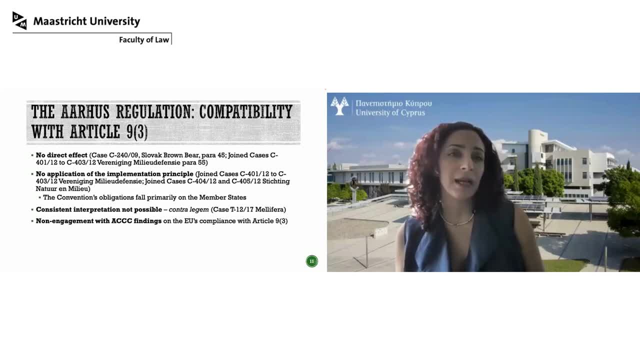 exempted by implementing laws. The fact that the Court was reluctant to rely on the interpretation offered by the review body tasked under international law with overseeing compliance with this agreement, I think raises questions as to the EU's strict observance of international law, while at the same time that we see the Court sort of trying to preserve political discretion. 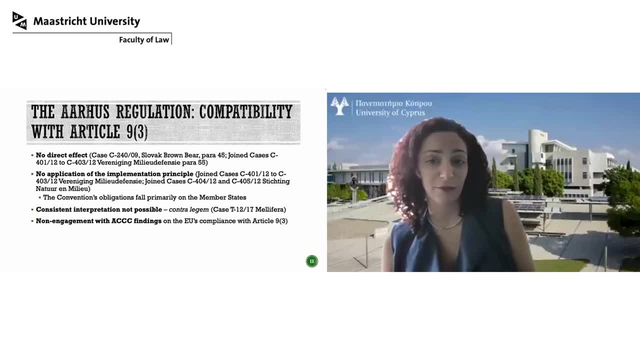 and allow the legislature to figure out the best way to comply with the ACC findings. So it's become clear that the solution would not come through judicial interpretation and the legislature was uh left to the option to change it, if they wish, by revising the regulation, which they did in 2021.. 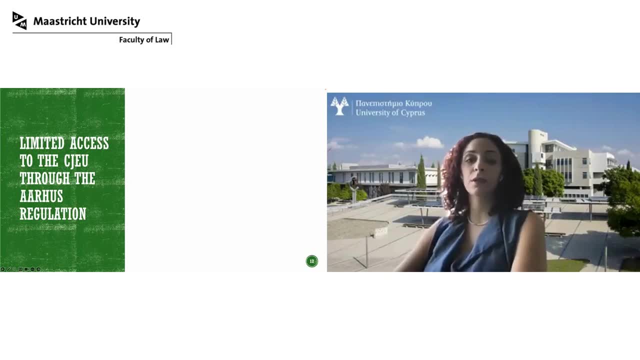 Now, before looking at the revised scope of the regulation, it is important to mention Article 12 of the AHU's regulation, which establishes a limited avenue of access to the Court for those environmental NGOs that have made requests under Article 10.. The ACCC had clarified that an interpretation of Article 12 that would limit judicial review to 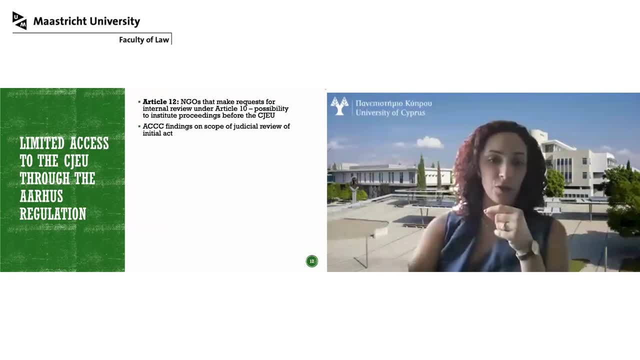 the written reply given by the institution to the NGO under Article 10 would be contrary to the requirements of the Convention. of the Convention. Nonetheless, the Court subsequently confirmed that it is limited or that Article 12 does not allow for the substance of the original Act to be reviewed by the Court. 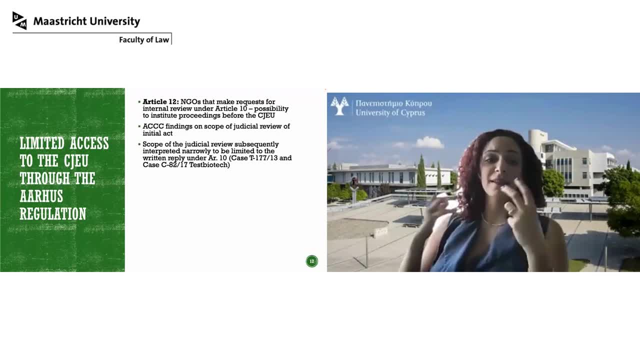 So this means that a successful application under Article 12 cannot lead to the annulment of the initial Act, which was challenged through Article 10, but only of the written reply that the institution gave to the institution, And so these documents must be reviewed. 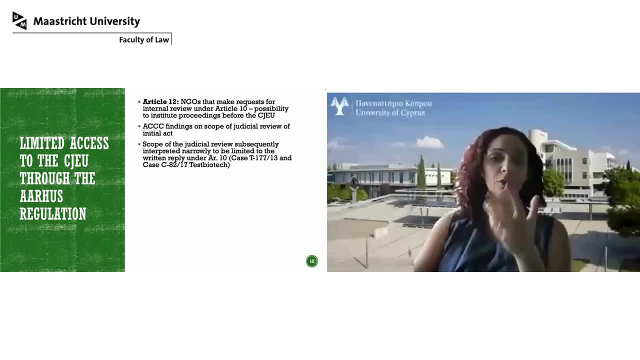 And these documents are not subject to the Act. In other words, there's no obligation to the report that the institution mentioned the NGO following the request under Article 10.. And the standard of review applied by the court is not very demanding. 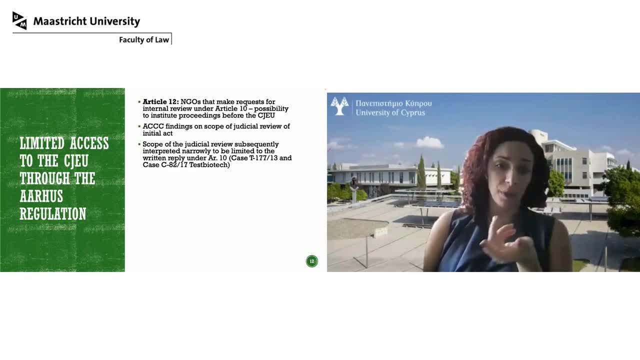 It examines whether the relevant institution committed a manifest error of assessment in its reply. Now, in practice, indirectly, grounds of review that were relevant in the request for internal review may be examined by the court, but no new arguments may be put forward. 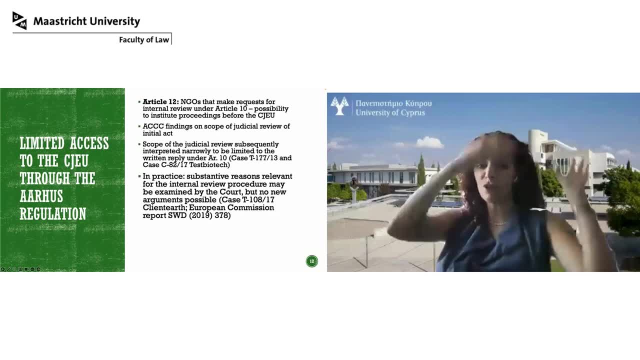 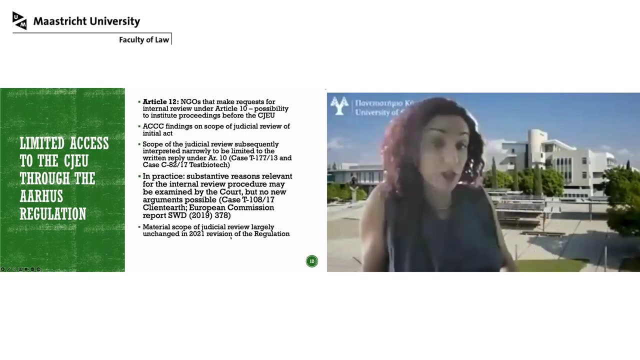 This effectively means that NGOs wishing to challenge the legality of the initial act can only use the annulment procedure for acts not addressed to them under Article 2634, according to which they are likely to have standing. as discussed earlier. Now the material scope of judicial review under Article 12. 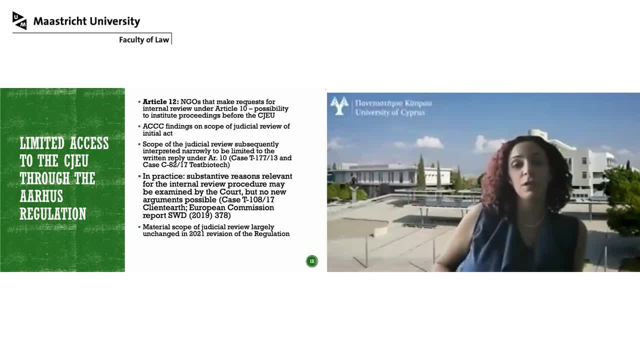 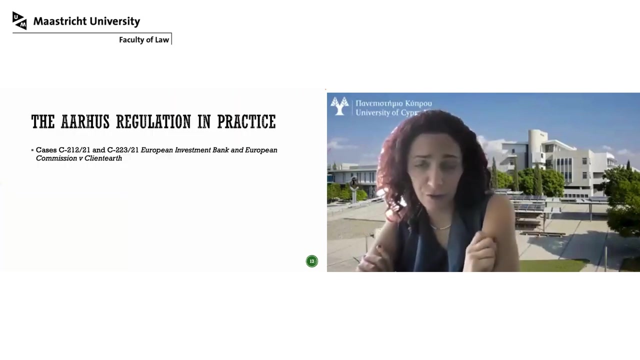 remains largely unchanged in the 2021 revision of the regulation, apart from a recital in the preamble clarifying that it covers both the procedural and substantive legality of the written reply. Now the scope of judicial review becomes clear when we look at the recent case. 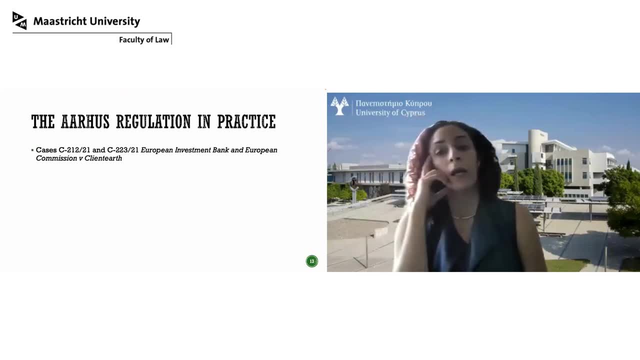 It's decided by the Court of Justice in July 2023, which demonstrates, I think, that despite its limitation, the ACWIS regulation offers promising accountability avenues. Now, this judgment concerns interpretation of the ACWIS regulation before its revision in 2021.. 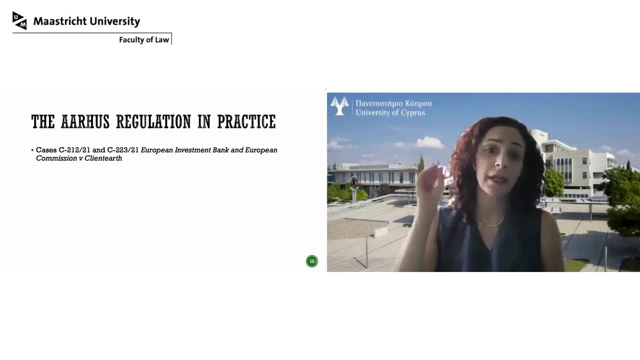 That's when the request was made, And it is likely, however, that the reasoning of the court was implicitly influenced by the subsequent broadening of the regulation. And it is likely that the reasoning of the court was implicitly influenced by the subsequent broadening. 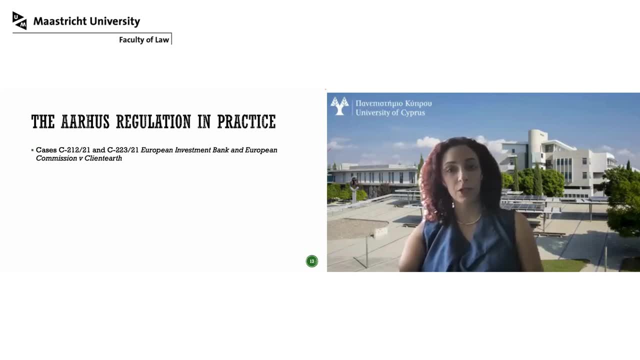 of the regulation. It is likely, however, that the reasoning of the court was implicitly influenced by the subsequent broadening of the regulation, That is that the result of the action of the regulation on the relevant grounds of the normative power of the European Union. 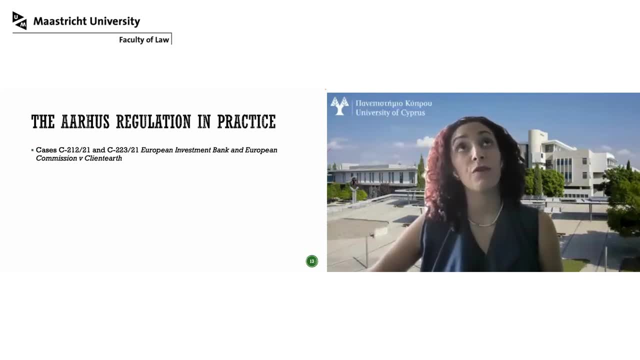 is still not clear. That is, the current position of the Commission on the Law on Environmental Refineration in Europe is teveberating. It is toward the same time we see what the Court of Justice has been doing to address its issue about the regulation of the ACWIS regulation. 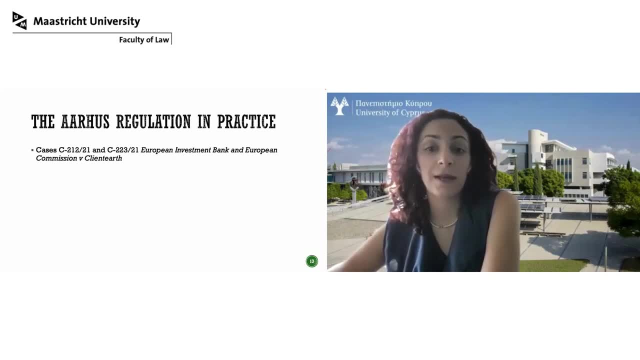 under Article 10 of Article 9 and Article 11 of Article 11.. The case concerns a request by an environmental NGO for internal review under Article 10 of a resolution by the Board of Directors of the European Investment Bank. the ground that it did not relate to an act amenable to internal review In terms. 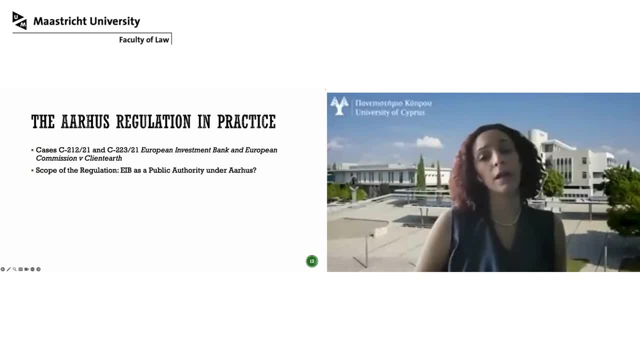 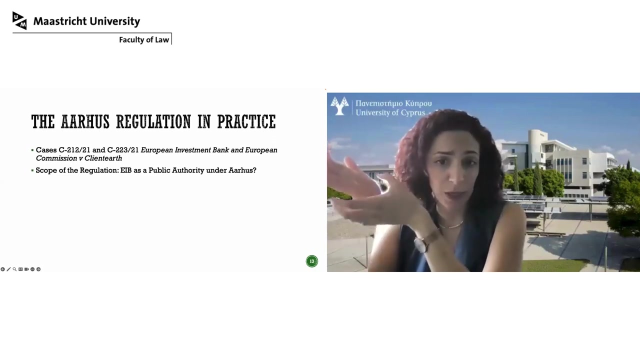 of the personal scope of the regulation. the court interpreted the regulation consistently with the Convention and clarified that only specific situations relating to a body acting in a judicial or legislative capacity or as an administrative review body under the treaty can be excluded. In the circumstances of the case, none of these exceptions applied Beyond its. 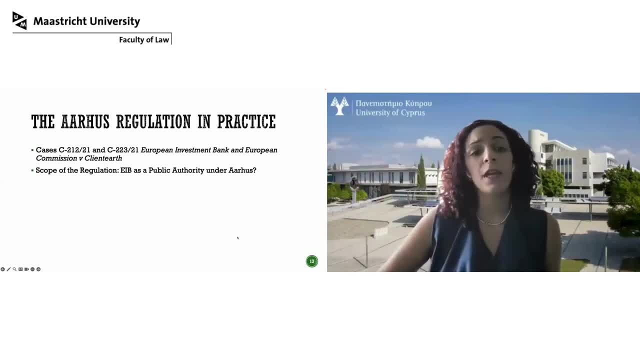 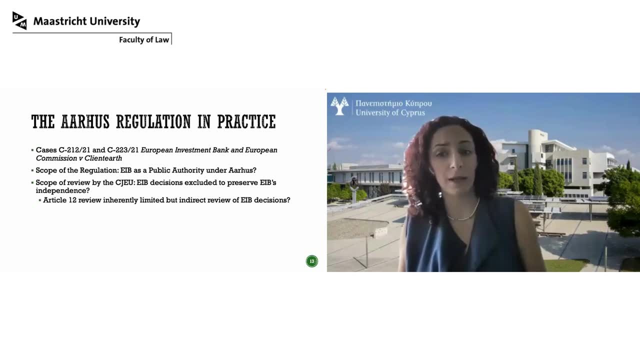 classification as a public authority. the EIB sought to limit the scope of the regulation by arguing that its refusal to the request by Client Earth was justified as a means to protect its independence on the financial markets. Now, Article 271, Paragraph 6, of the EIB states that the EIB should not be. 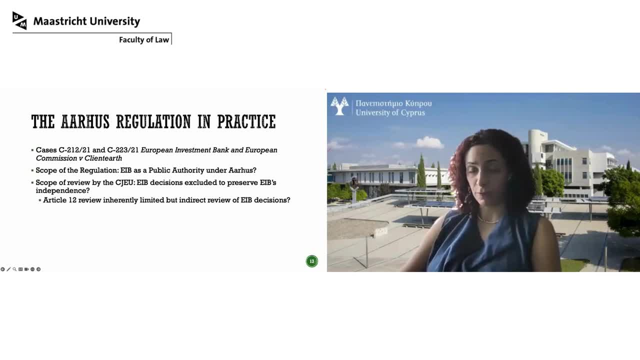 subject to the strict conditions that the Containment and Discipline Act for its purpose sets out. The EIB's measures also attempt to put in place a strict thing of the EIB's board of directors, both in relation to the applicants that can bring such actions. 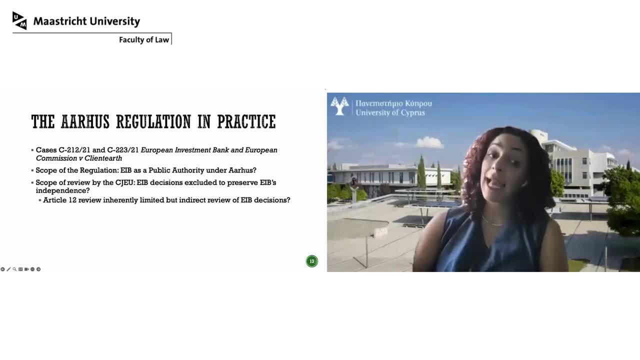 and in the scope of the EIB's review, which is limited to grounds of non-compliance with procedures set out in the EIB's Statutes, None of these conditions have been. Nevertheless, according to the court, this provision- Article 271, cannot limit the indirect 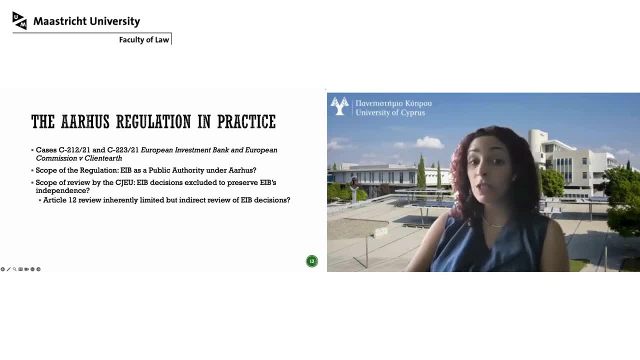 review of EIB resolutions by the court, nor deprive environmental organisations from the right to request an internal review under Article 10 of the ARCUS Regulation and the corresponding right to bring an action for annulment against a decision requesting the request under Article 12.. 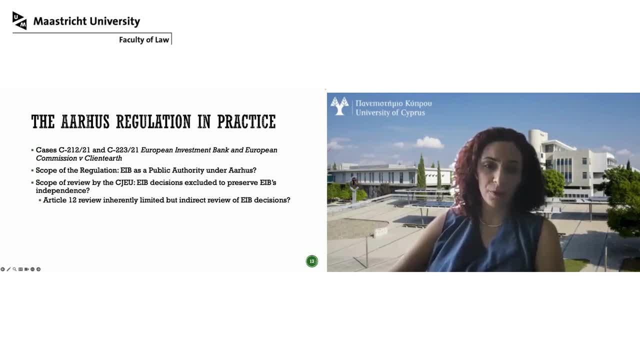 In essence, the application of Article 12 of the ARCUS Regulation to EIB resolutions does not directly expand the court's jurisdiction over EIB measures, as its review can only lead to a decision requesting the EIB to internally review the resolution itself, and not to its 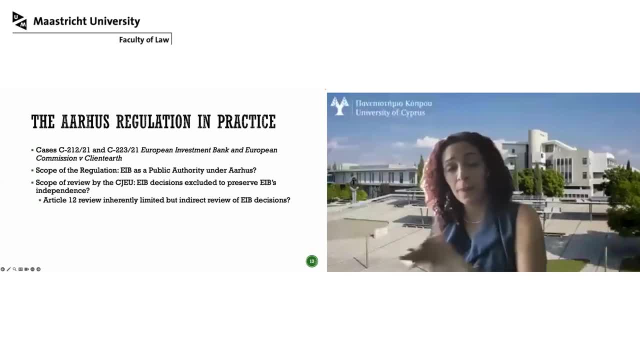 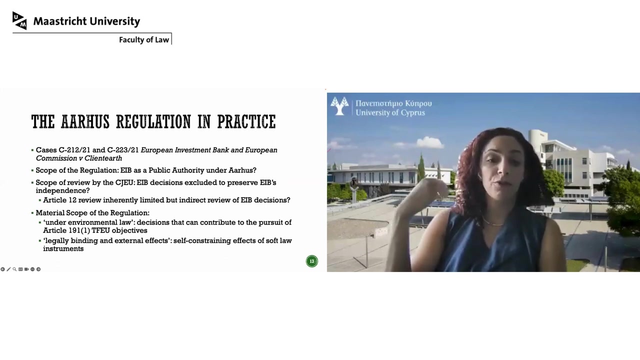 annulment by the court. As we saw earlier, Article 12 review cannot lead to the annulment of the initial act. Finally, regarding the material scope of the regulation, both the Court of Justice and the General Court adopted the teleological approach of the requirement for an act to 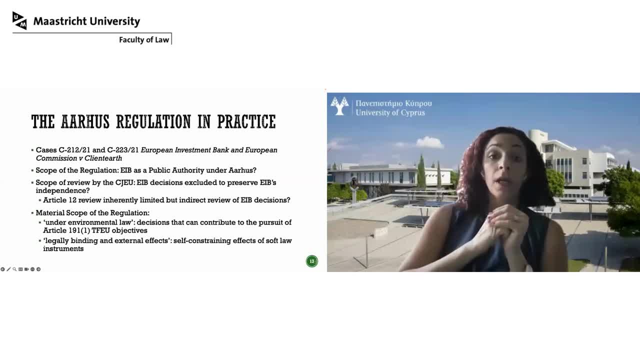 be adopted under environmental law. The ARCUS Regulation, according to the Court, covers acts which can infringe environmental law. In this context, the EIB's climate strategy and the statement of environmental and social principles and standards which require the EIB to take into account environmental criteria. 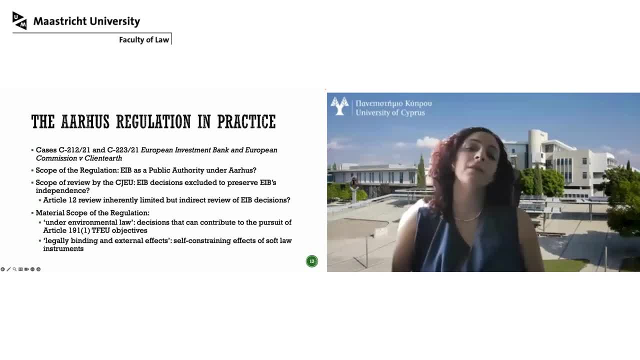 in determining the eligibility of projects rendered the decision taken under environmental law. 1. This approach reflects the clarifications in the 2021 revision of the regulation, which cover acts adopted in the implementation of other non-environmental policies which should be subject to internal review. In this context, the court indicated that: 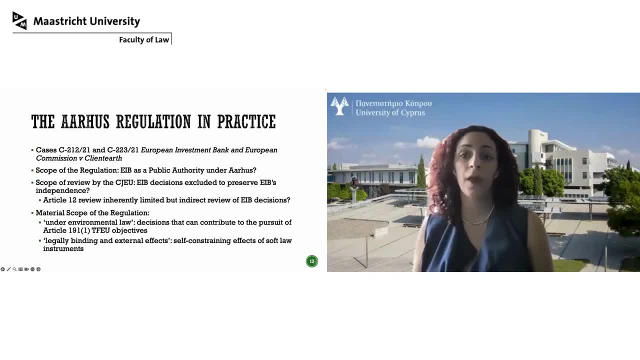 when taking lending decisions, the EIB cannot without justification depart from the environmental criteria it set for itself in the Climate Strategy, in the 2009 Statement of Environmental and Social Principles. So it held that the EIB cannot unjustifiably depart or ignore this criteria. 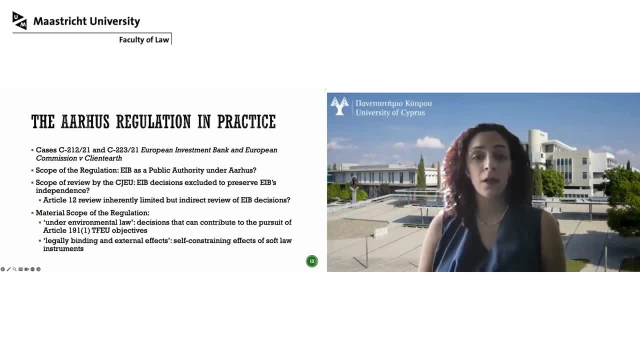 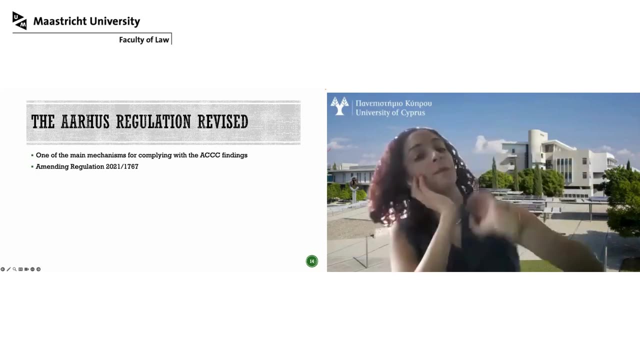 without risking violating the principle of equality. Now moving to how the regulation was actually revised in 2021.. Following the ACC findings against the EU for restrictive access to the court, the Commission and the Council stressed that they could not indicate to the Court of Justice how to 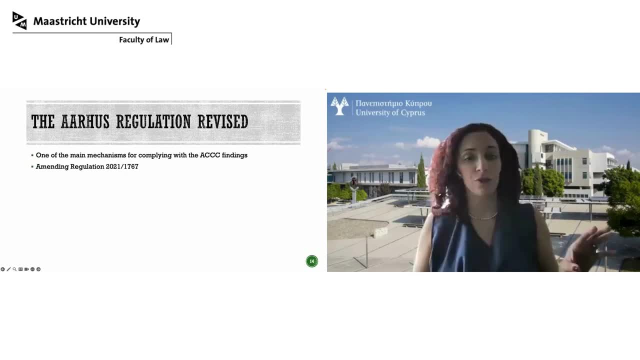 interpret Article 263. Separation of power is the doctoral view and judicial interpretation is the exclusive jurisdiction of the Court. Instead, one of two ways for ensuring compliance with the ARIFAS Convention was to expand the scope of the ARIFAS Regulation, which they did in 2021.. In terms of its personal scope, A significant step. 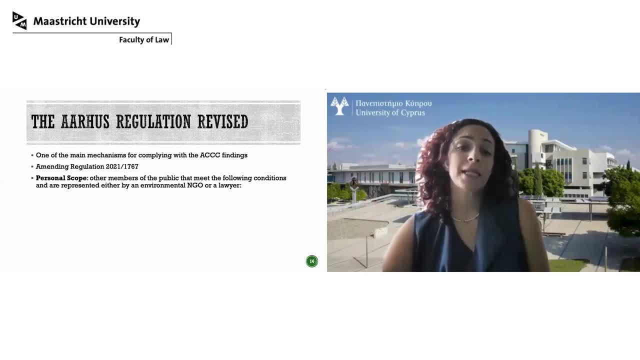 was achieved by the European Parliament and Council, by the EIB's collaboration with EIB's national, so by extending beyond NGOs to members of the public, in two instances. The first is determined by qualitative criteria, when there is impairment of rights caused by the alleged contravention of environmental law and when members of the public are directly. 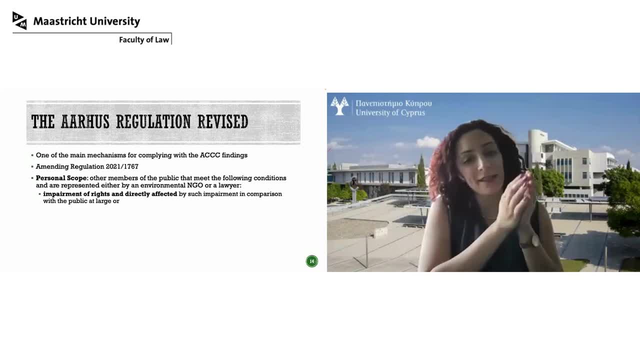 affected in comparison with the public at large. Directly affected is not the same as individual and direct concern under Article 2634.. This means that they are directly affected in comparison with the public at large, for example, in the case of an imminent threat to their own health or prejudice caused to. 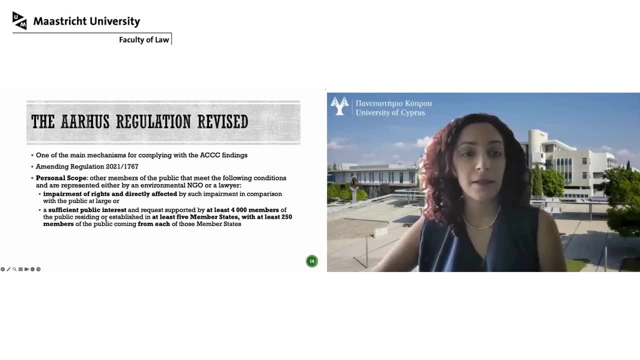 a right that they are entitled to under the law. The second instance is a combination of qualitative and quantitative criteria, When there is a sufficient public interest in protecting the environment, human health and so on, which is proven collectively, as the request has to come from a minimum number. of members of the public: 250 members of the public at least, from a minimum number of member states. 4,000 members of the public, that's the minimum for the whole country. That's a collective sort of move, And then 250 have to come from each of five member states. 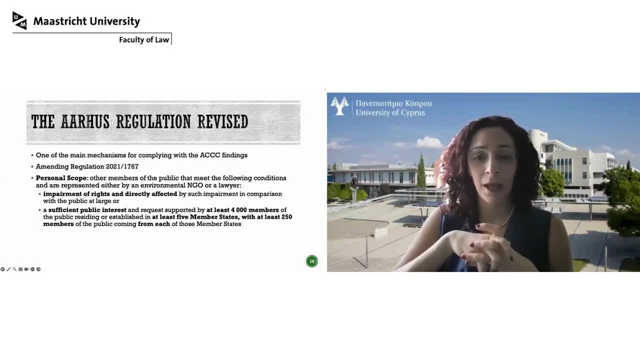 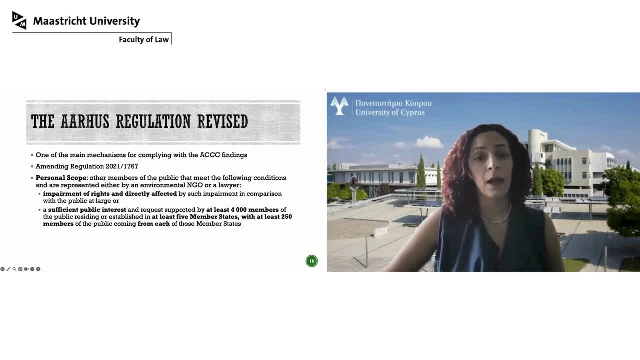 There was some sort of delay in allowing time to the administration to adapt to this broadened scope. And, apart from the personal scope, the material scope was also extended and this came in force already in 2021.. Extending now beyond acts of individual scope and beyond acts adopted under the environmental 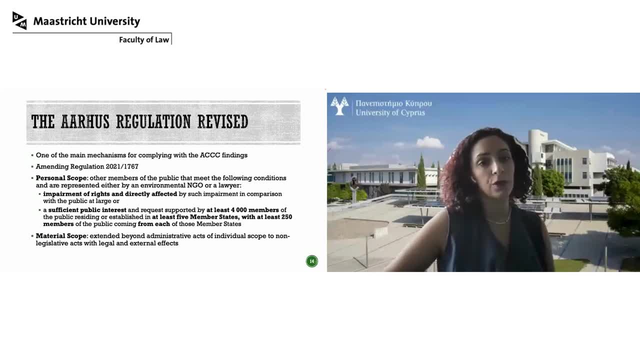 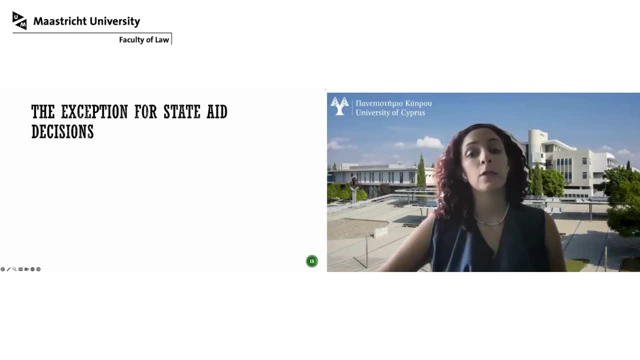 legal basis, which essentially covers a larger portion of requests Extending now beyond acts of individual scope and beyond acts adopted under the environmental basis, which essentially covers a larger portion of requests Extending now beyond acts of individual scope and beyond acts adopted under the environmental 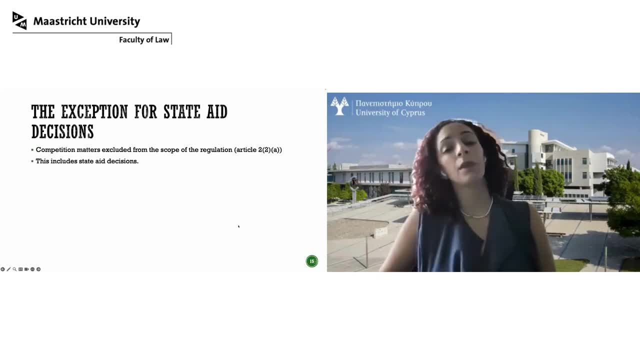 law, it places itself at a very significant height. Yet still, the material scope excludes commission decisions on state aid which may contravene environmental law. as provided in article 2 of the regulation, Statate decisions can be powerful instruments that affect the environment. 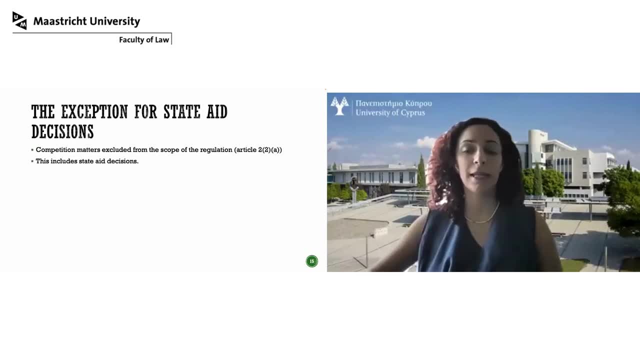 They shape the EU's energy markets. they determine support to fossil fuels, renewable energy sources and can have a direct impact on the balance between polluting and non-polluting, and they shape the EU's energy markets. This is not the case for sustainable energy. 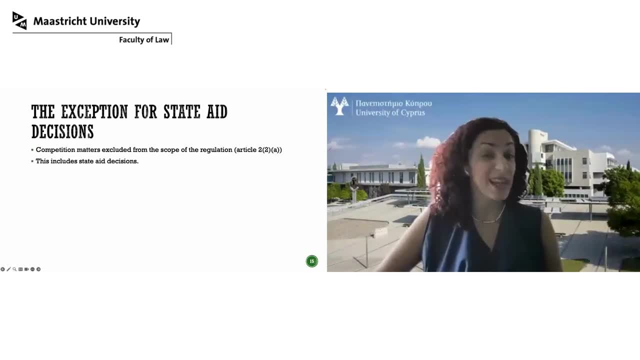 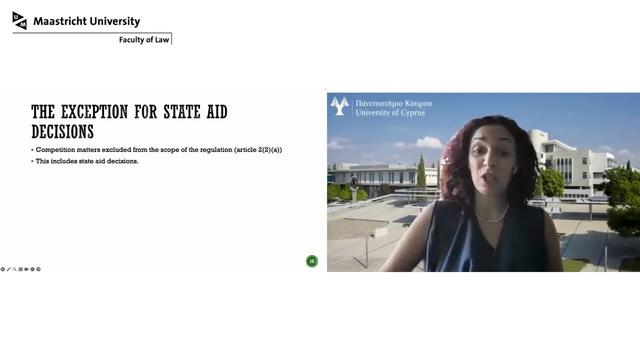 to challenge the compatibility at EU level. Their exclusion from the scope has no basis in the Aarhus Convention, which only excludes acts adopted by public authorities acting in legislative or judicial capacities. In March 2021, the ACCC found against the EU for failing to provide access to justice. 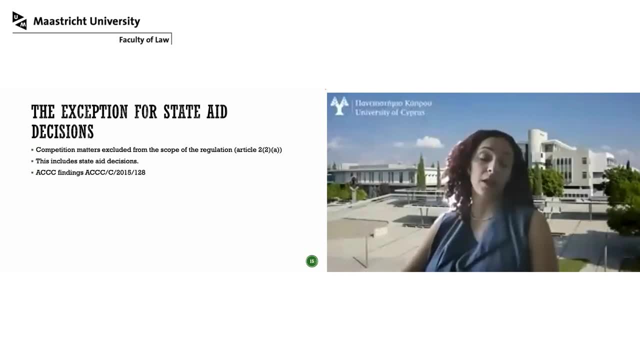 to environmental NGOs against Commission-stated decisions recommending that EU law should be changed With pressure from the EU. the meeting of the parties to the Aarhus Convention in its findings to the next meeting in 2025, basically, until the EU figures out how to comply with. 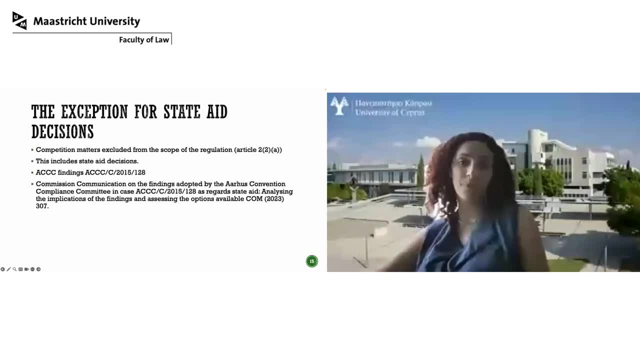 the findings In May 2023,. following a public consultation, the Commission issued a communication which stresses that ensuring compliance with these ACCC findings requires an adjustment to the existing legal framework or an equivalent measure, And in the communication, We have two key objectives. 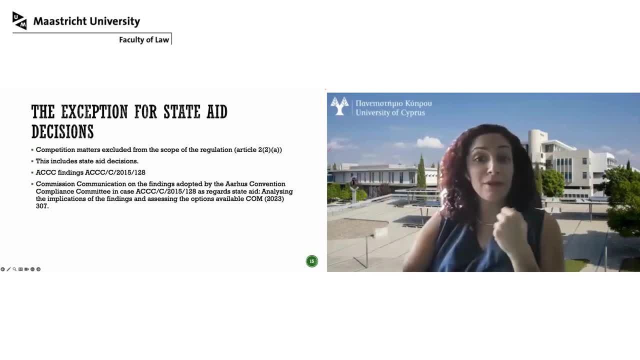 On the one hand, ensuring compliance with the Aarhus Convention and, on the other, preserving the specificities of state aid control and its effectiveness as one of the tools that can speed up the green transition. How to find a balance between the two is something that the Commission is currently considering. 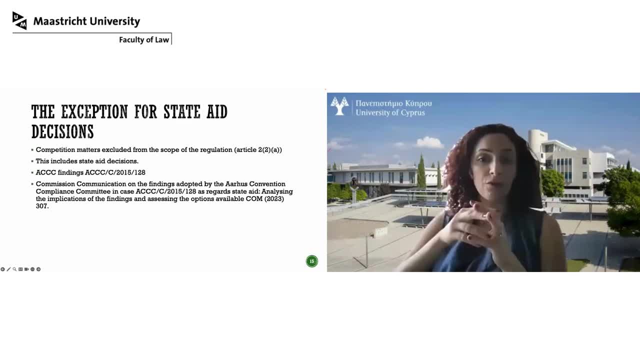 It's considering different options, including amending the Aarhus regulation to include state aid decisions, But of course we should bear in mind that an administrative act that would be reviewable under the Aarhus regulation comes only at the final stage, once the decision actually 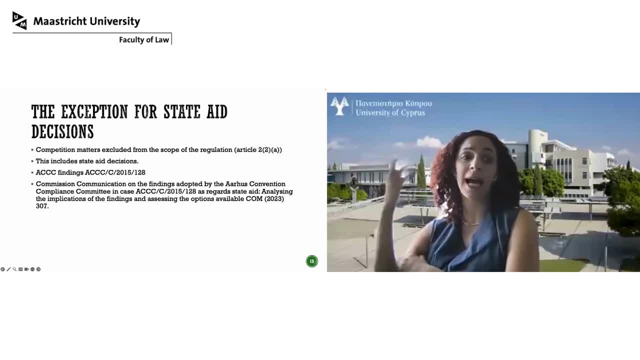 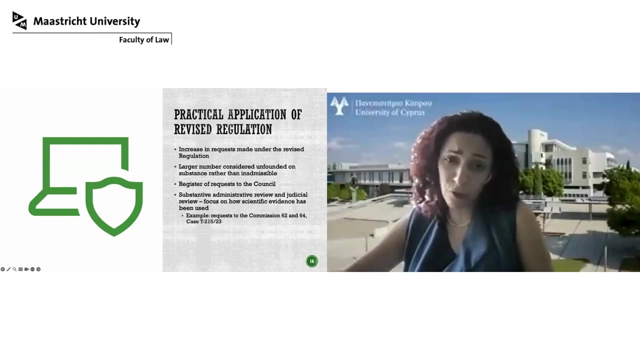 exists in state aid proceedings, So it remains to be seen how, and to what extent state aid decisions will be reviewable. Now, what is the broadening scope of the regulation, And will it be sufficient to fill the gap and meaningfully comply with the Aarhus Convention? 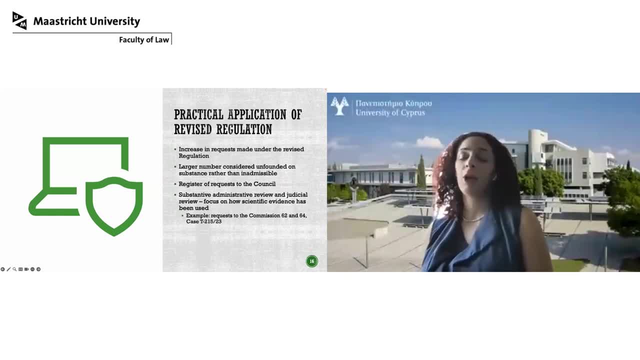 Remains to be determined in practice, But we do have some trends already visible that are quite telling. Before the revision of the regulation, we had 48 requests with the Commission since its entry into force in 2007.. After the revision in 2021, we have an additional 33 requests. Demonstration of the Aarhus Convention is ongoing. The Aarhus Convention has been in force since 2007.. We have an additional 33 requests. Demonstration of the Aarhus Convention has been in force since 2007.. We have an additional 33 requests. 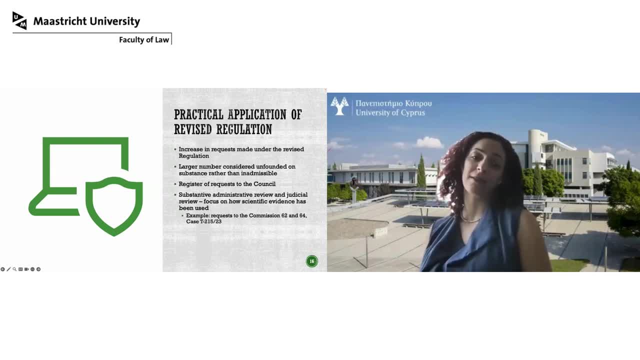 Demonstrating an important increase in requests now that generally applicable acts are reviewable. Also, comparatively with pre-revision requests, a larger number are considered unfounded on substance rather than deemed inadmissible. So overall there is more of a balance between unfounded and inadmissible requests at the 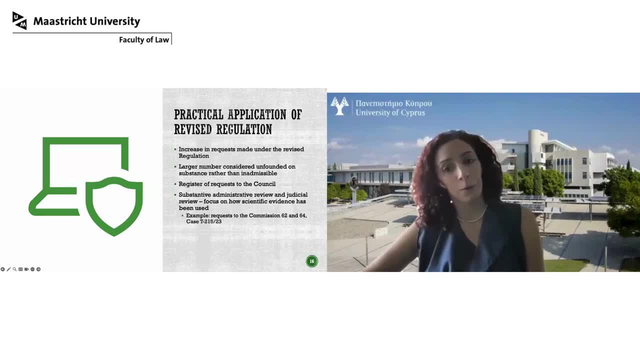 moment. For example, a review request of the fourth union list of projects of common interest, which are key cross-border energy infrastructure projects, was previously found inadmissible by the Commission. New lists from the fifth, published in November 2021, always are now reviewable. 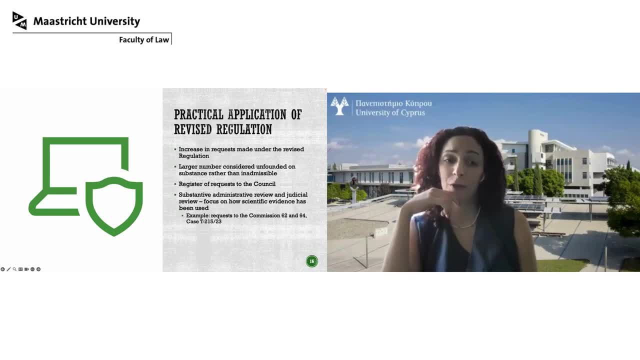 We also have review requests to the Council, which now has an established public registry, which is an area of decision subject to review by the Council yearly, concerning regulations fixing fishing opportunities, the so-called total allowable catches under the common fisheries policy. The focus of the substance reviews and of the judicial review under Article 12 seems 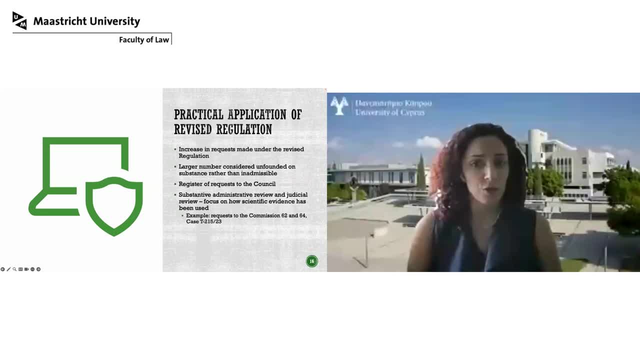 to be on how relevant scientific evidence is being used by institutions. So applicants and NGOs frequently ask questions. They frequently argue that the institution adopted an act breaching environmental law because it has not sufficiently relied on the latest scientific evidence, the precautionary principle and so on. 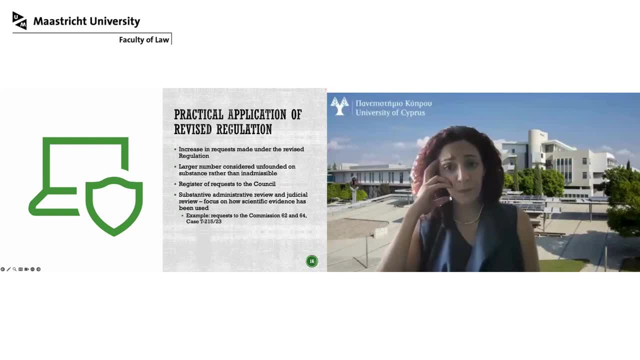 To give you an example that is quite important. two requests were made concerning the Commission's classification of energy source from biomass, From forest biomass, as sustainable. under the EU taxonomy for sustainable finance regulation, The Commission relied on the classification of forest biomass as a renewable energy source. 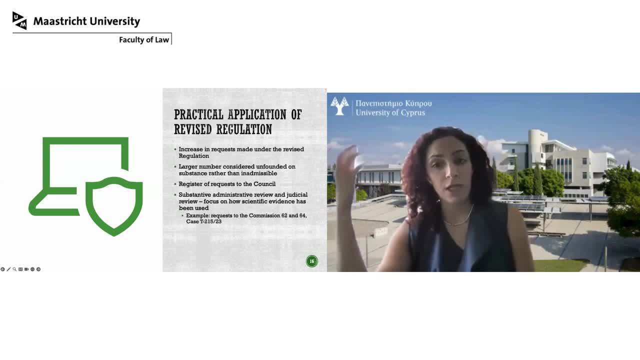 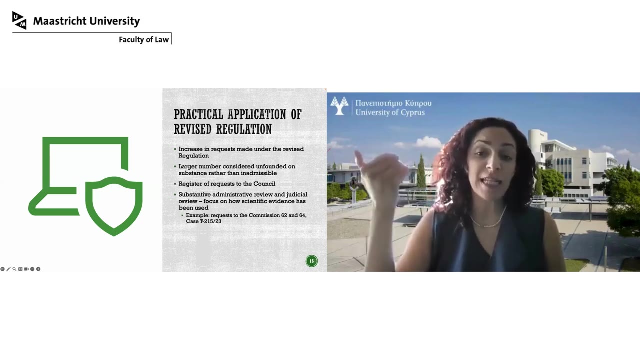 in EU legislation, according to the NGO, without taking into account the most recent evidence showing the high level of greenhouse gas emissions incurred by burning forest biomass, And to this effect a case was launched in April 2023, challenging the Commission's reply. 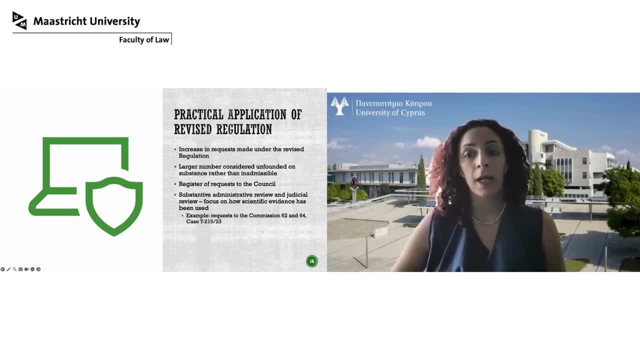 and its assessment to the NGOs. Now it remains to be seen how the General Court will decide, but we should recall that it sets out case law that EU institutions have a wide margin of discretion in assessing scientific evidence, which is often quite complex. Judicial review is limited to examining whether or not the EU institutions have a wide margin. 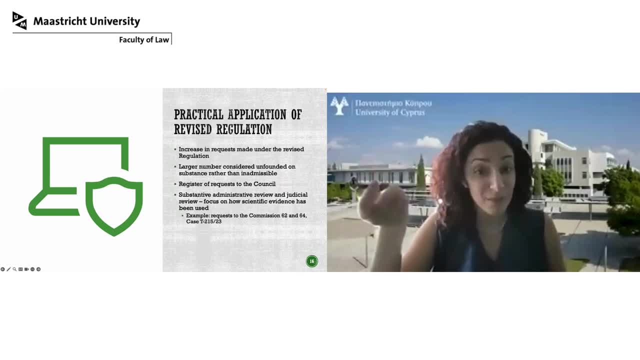 of discretion in assessing scientific evidence, which is often quite complex. Judicial review is limited to examining whether or not the EU institutions have a wide margin of discretion in assessing scientific evidence, which is often quite complex. Judicial review is limited to examining whether or not the EU institutions have a wide margin. 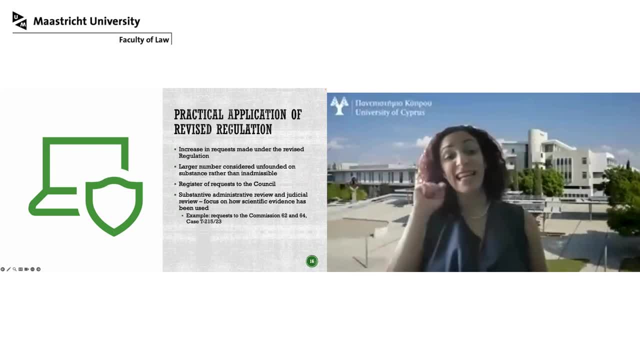 of discretion in assessing scientific evidence, which is often quite complex. Judicial review is limited to examining whether or not the EU institutions have a wide margin of discretion in assessing scientific evidence, which is often quite complex. Judicial review is limited to examining whether or not the EU institutions have a wide margin. 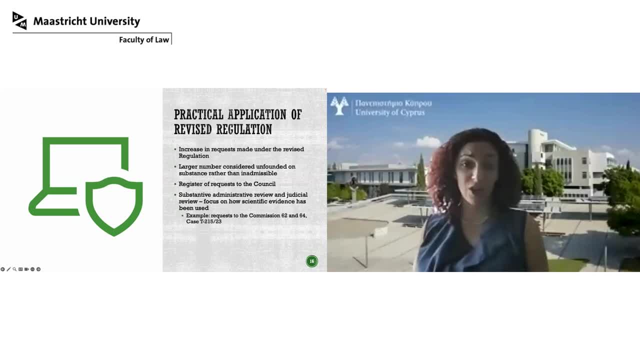 of discretion in assessing scientific evidence, which is often quite complex. Judicial review is limited to examining whether or not the EU institutions have a wide margin of discretion in assessing scientific evidence, which is often quite complex. Judicial review is limited to examining whether or not the EU institutions have a wide margin. 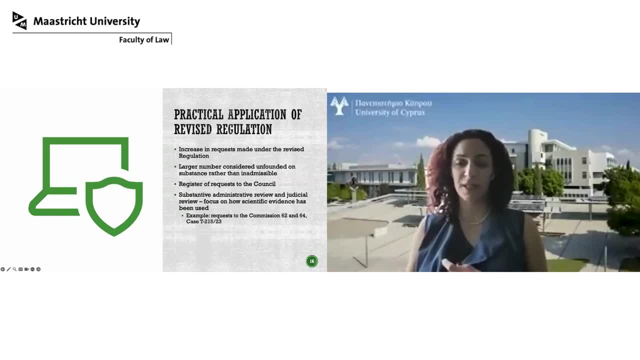 of discretion in assessing scientific evidence, which is often quite complex. Judicial review is limited to examining whether or not the EU institutions have a wide margin of discretion in assessing scientific evidence, which is often quite complex. Judicial review is limited to assessing scientific evidence, which is often quite complex. 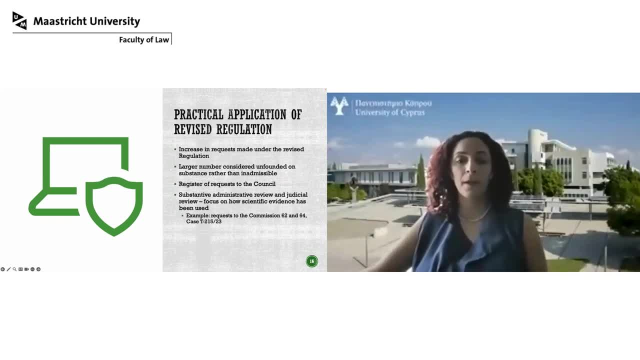 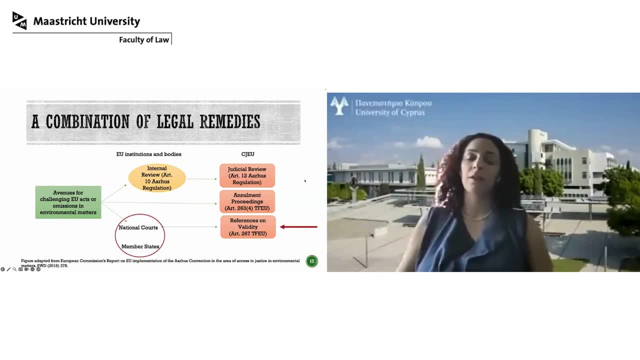 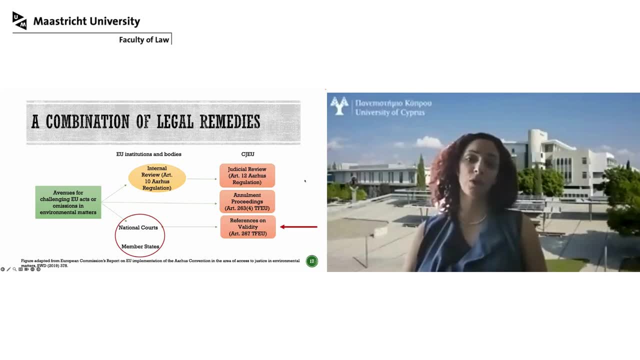 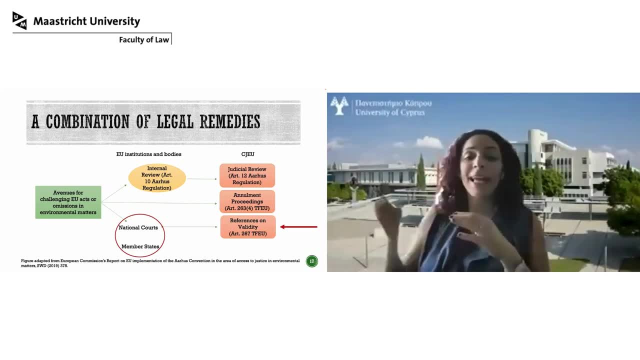 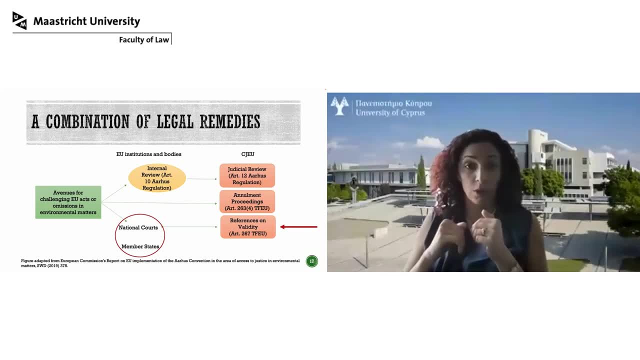 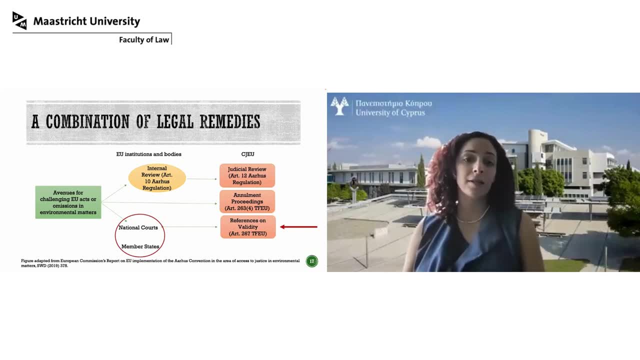 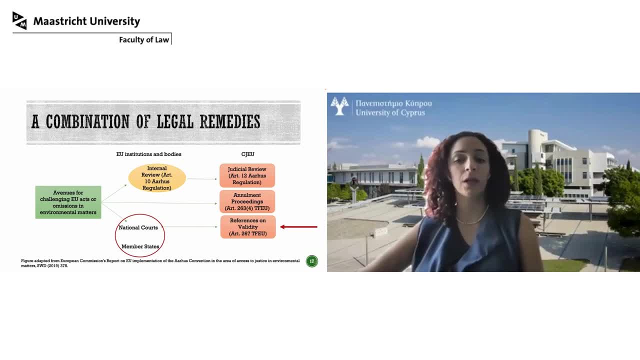 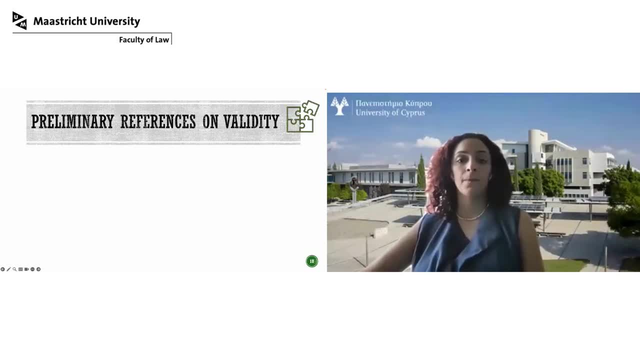 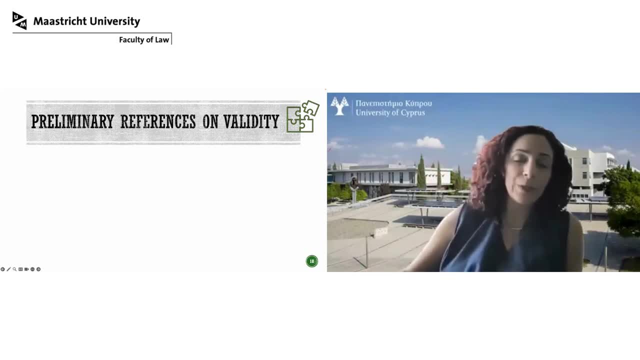 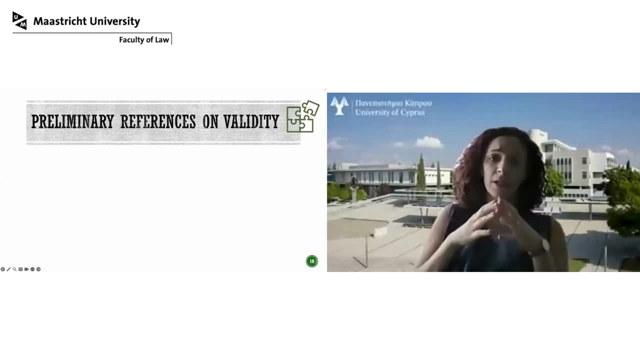 If the national court is inclined to find the validity challenge well-founded, then it has to send preliminary questions to the Court of Justice, which has exclusive jurisdiction to review the legality of EU Act. However, a national court may decide that it is not necessary to refer and instead hold that the EU Act is valid. 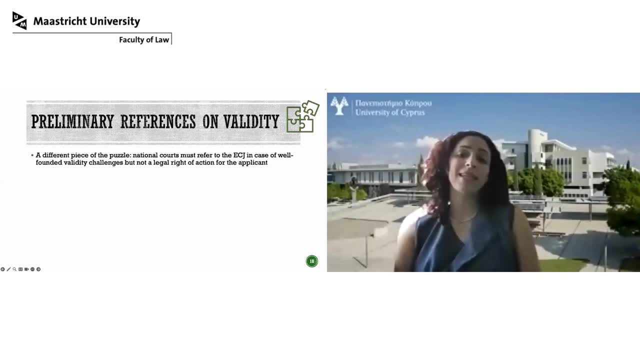 So this means that this request mechanism is an inherently different piece to the puzzle. It is not a legal right of action for the applicant, who may ask the court to send questions to the Court of Justice, but it is ultimately a judicial decision whether to do so. 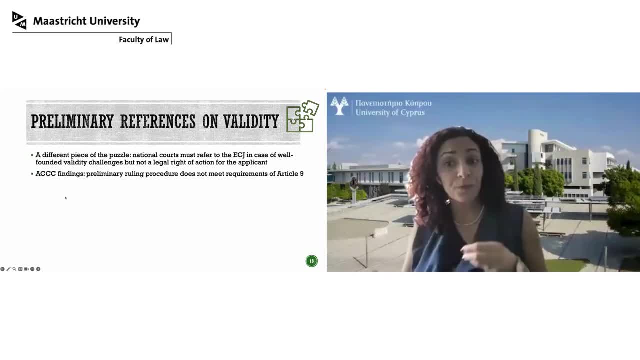 In light of these concerns, the ACCC has ruled that it does not meet the requirements for securing the rights of Article 9.3 and does not compensate for the restrictive access to the Court directly under Article 2634.. Of course, there are many benefits to accessing national courts. 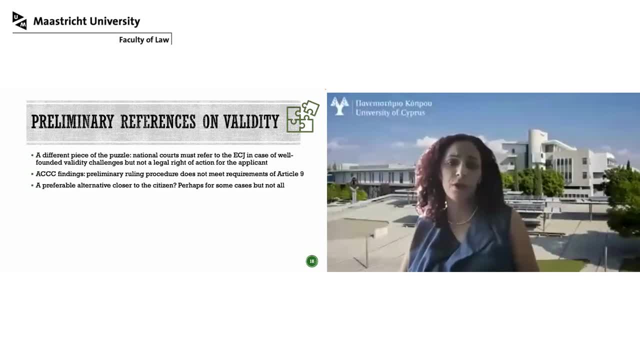 The familiarity of applicants with the system, the language used. it is closer to the citizens For certain situations, for example involving violations of environmental law by national authorities, authorisation of individual projects in member states, But when it is about the legality of EU technical 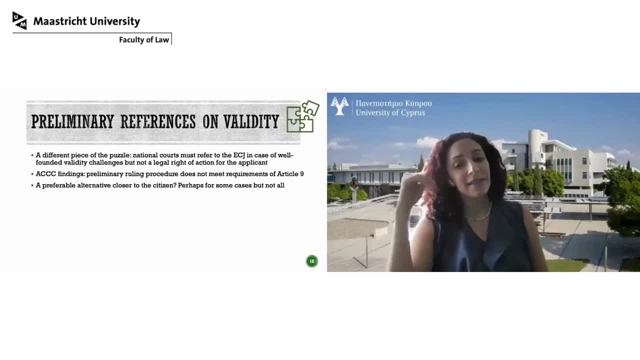 and politically charged acts. access to the court of justice directly and throughout the whole cycle of the case is preferable as it involves a critical role by the general court and ensures a uniform system of review for violations by EU institutions that does not depend on procedural rules. 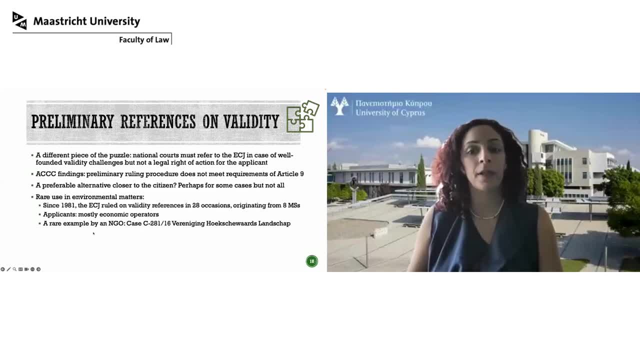 of different member states. In any case, to date this avenue has not served a significant role in environmental cases. It's made a minimal contribution. Since 1981, we have about 28 occasions of preliminary references on validity in environmental issues. 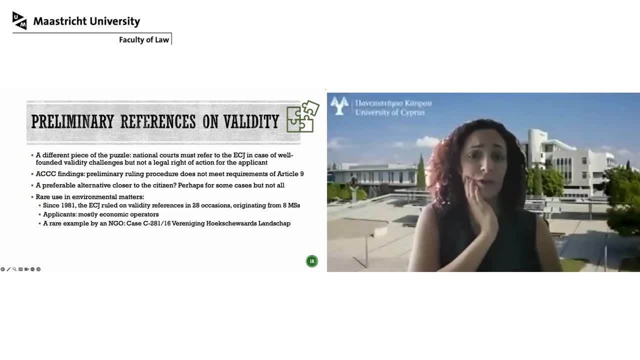 Coming from eight member states and usually involving economic operators as the applicants. We have one rare example by an environmental NGO, which is also one of the rare instances, which led to the annulment of the Commission decision And this considered the decision of the Commission. 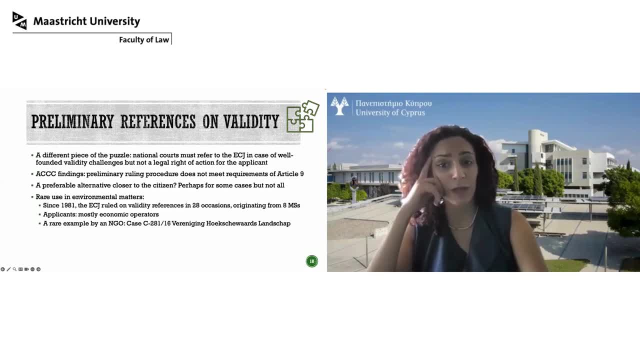 to authorise amendments to the list of sites of community importance under the Habitats Directive to reduce the size of a special area in the Netherlands. Overall, it is the less frequently used mechanism, both compared to the AHRQ's regulation and Article 2634.. 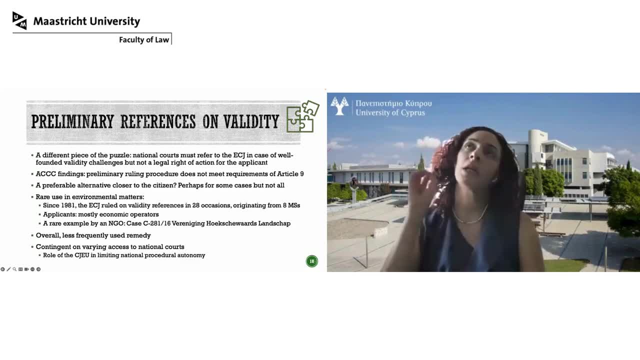 This may be partly explained by the reluctance of national courts to send preliminary questions on validity, And we should bear in mind that its use is also contingent on varying standing requirements for accessing national courts in the first place. On this front, the Court of Justice has played a crucial role. 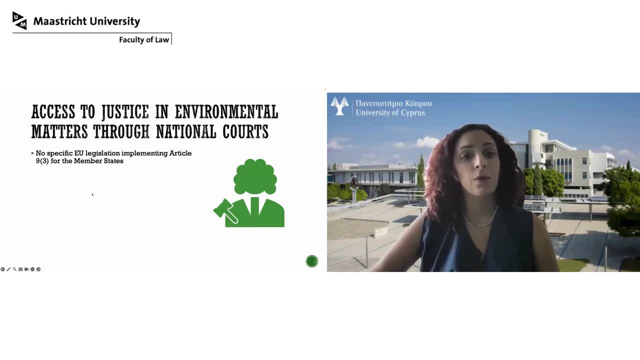 Even though we do not have specifically EU secondary legislation implementing Article 93 for the member states. Outside of areas where we have EU secondary legislation, the starting point is that member states have procedural autonomy subject to national law, So this is a very important point. 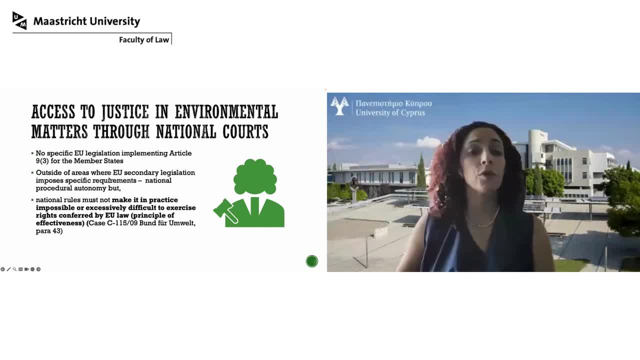 It is a very important point. We need to consider the possibility of international remedies not making it in practice impossible or excessively difficult to exercise rights compared to the EU law. In this context, partly on the basis of Article 93 of the AHRQ Convention, 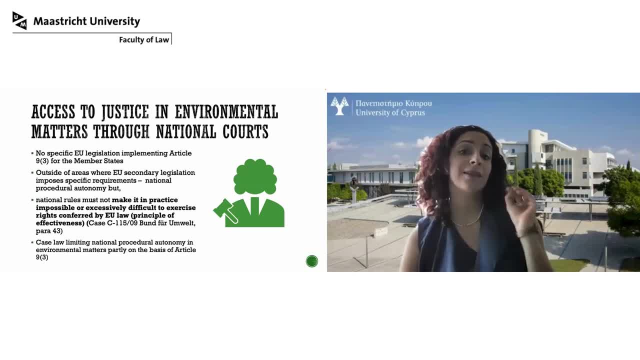 and partly on the basis of EU law principles, the Court has limited procedural autonomy in environmental matters to ensure wide access to justice, especially for environmental NGOs, as Professor Marjolina Eliantonio will examine in next month's lecture, So I will leave that point there. 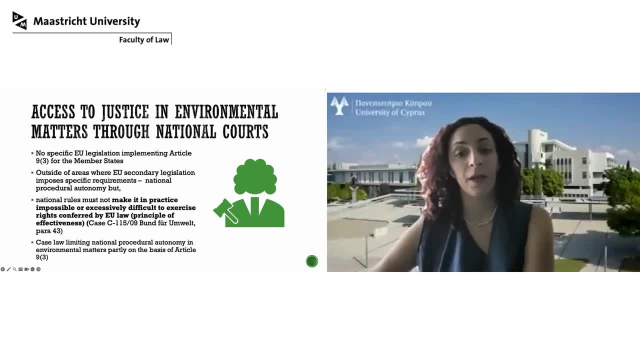 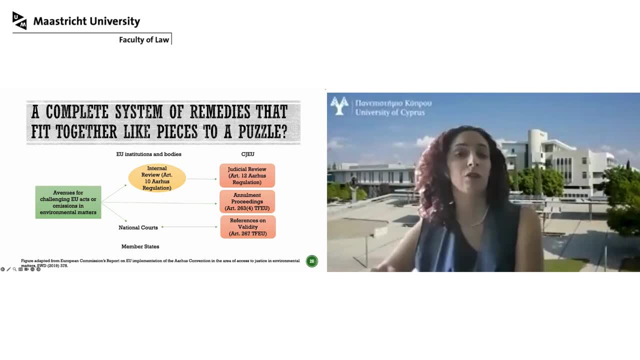 and it will be further explored in next month's lecture. So overall, to conclude, the Court seems to insist on its long-standing rationale that effective judicial protection for environmental matters will be ensured through a combination of the following principles. The first principle is that the legal system 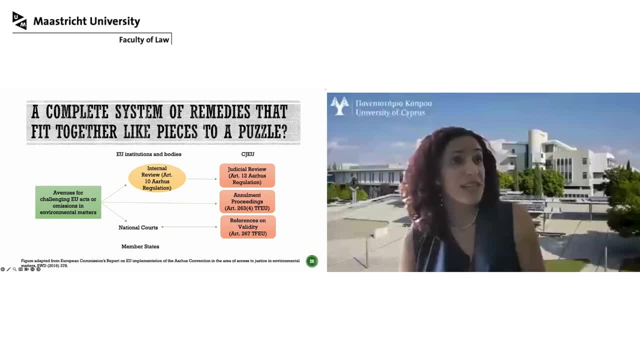 must be designed to be a system of legal remedies that together amount to a complete system. Interestingly, it also seems to have thrown the ball to the treaty makers, reiterating that it is up to the Member States to revise the current system of remedies. 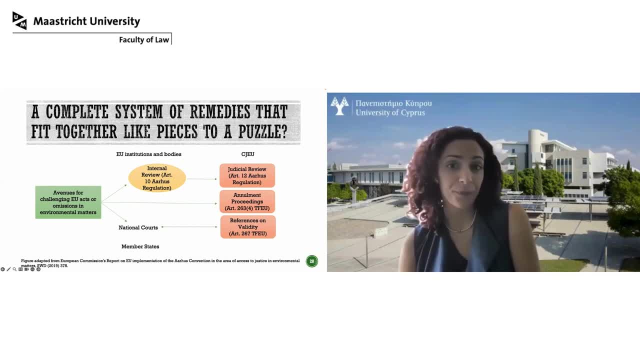 possibly by creating an environmental avenue of access to justice under the treaty. Until then, the alternative avenues under the AHRQ's regulation and access to national courts, which can lead to preliminary references on validity, remain pivotal Preliminary references on validity. 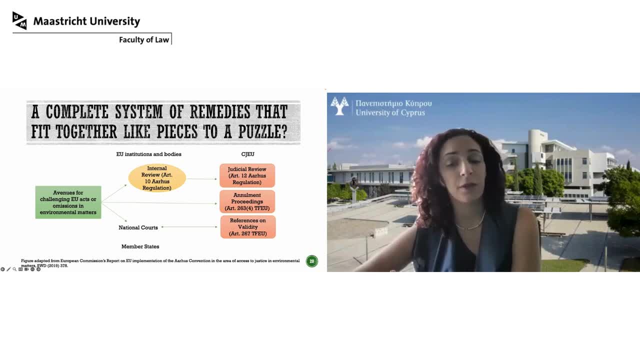 in light of their different nature as a mechanism and the rare use in practice, do not seem to offer the panacea to the EU's shortcomings for guaranteeing access to justice that both the Court and the Commission make it out to be Ensuring that procedural rules in the 27 Member States. 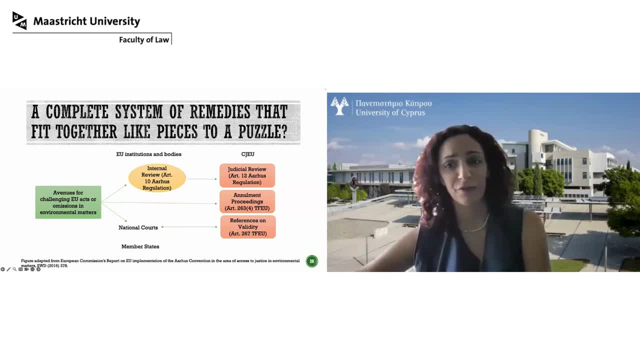 do not preclude access to the national court, which can then lead to a preliminary reference on validity, will not happen overnight, And within this context, the importance of the AHRQ's regulation as a key piece to the puzzle of legal remedies becomes even more visible.